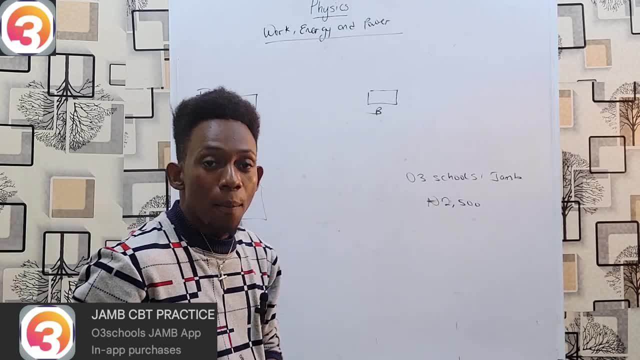 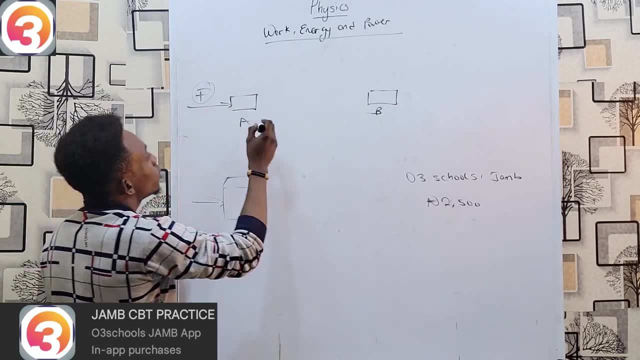 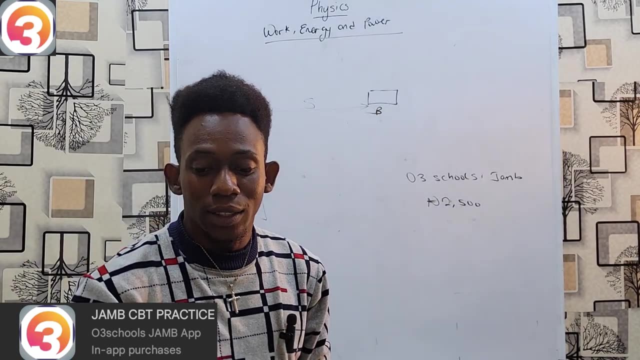 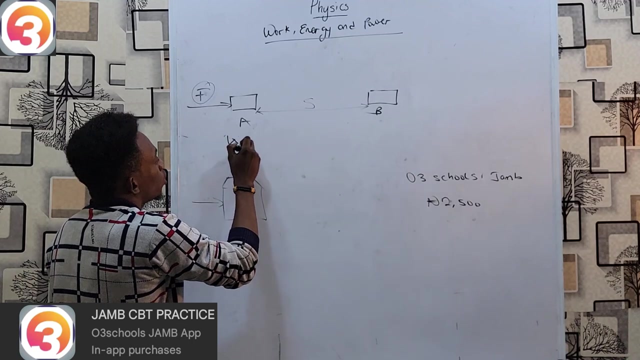 which obviously would not move. then my work done in that case will be zero. because for what to be done there are two agents necessary: force and a distance. if there is no distance, then there is no true work being done, because mathematically, work done equals to work done equals to force times distance. so that is that your distance is zero, zero times. 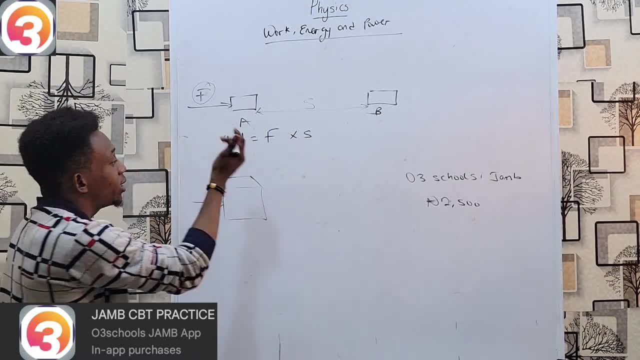 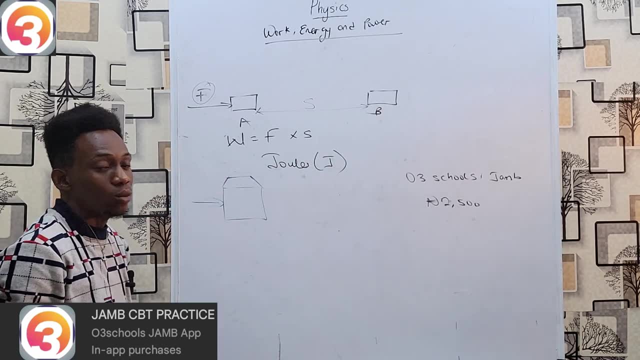 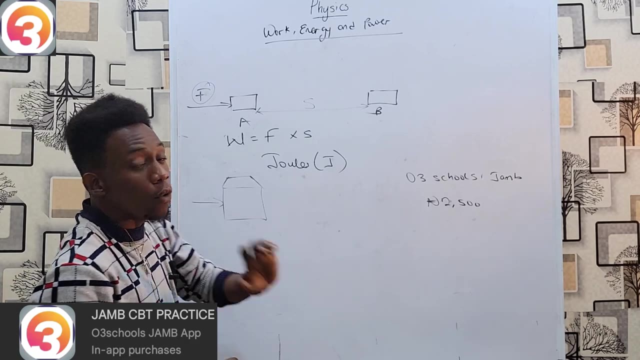 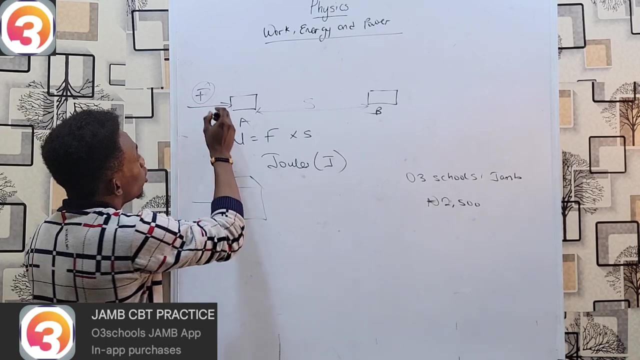 anything returns a value of zero. so the unit of work is jose j-o-u-l-e-s short form, calculator j, and work is a scalar quantity. that's that for work. and please note, the force being applied and the distance being moved in must be parallel to each other. that means if my force is horizontal, my distance will also be. 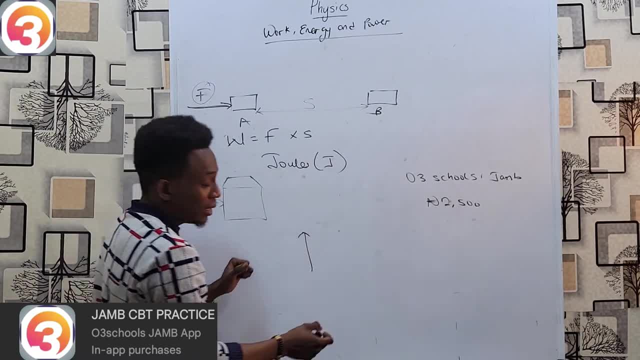 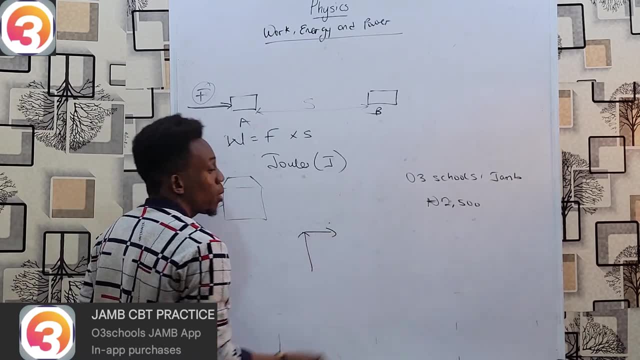 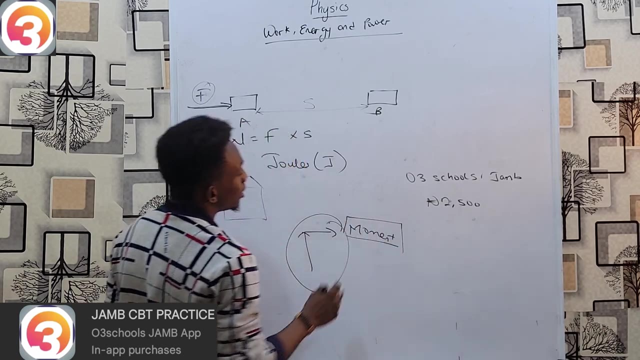 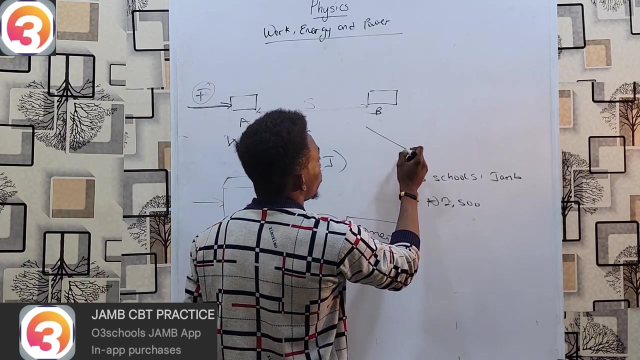 horizontal. if my force is vertical, then my distance- the object is moving- must also be vertical. if your force and your distance happen to be perpendicular, then this is moment which actually exists. in a totally separate topic. you try not to mix. it's work now. reason why this is important is that at times, your force will act on your object at an angle. 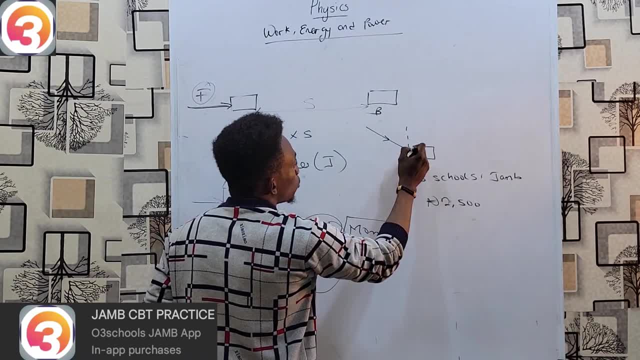 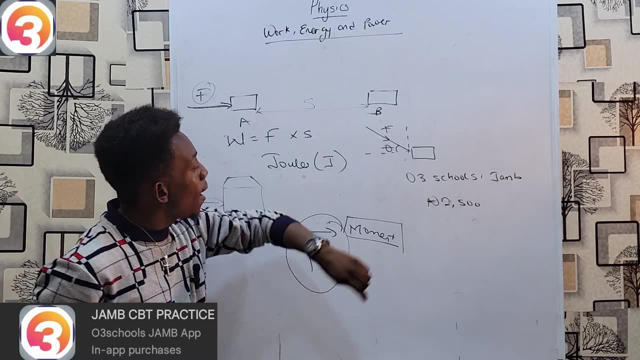 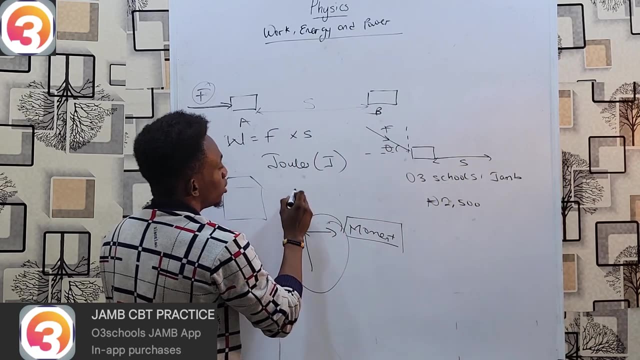 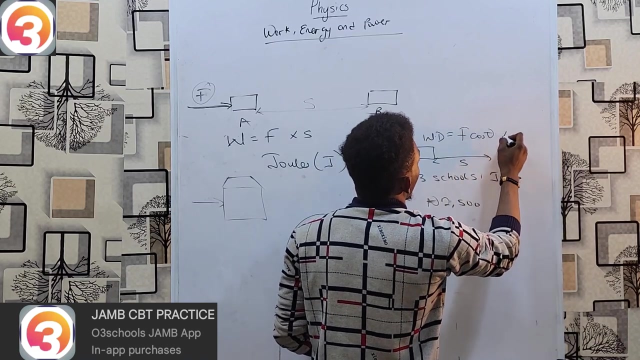 say, my force is acting here at this angle theta. in that case i can't just use my force on the zone, i have to resolve it to the horizontal component so that i can match my horizontal displacement and therefore my work done in this case becomes f? cos theta times s. now that is a basic and very 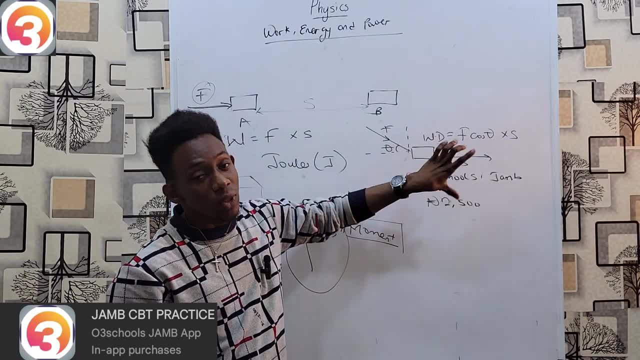 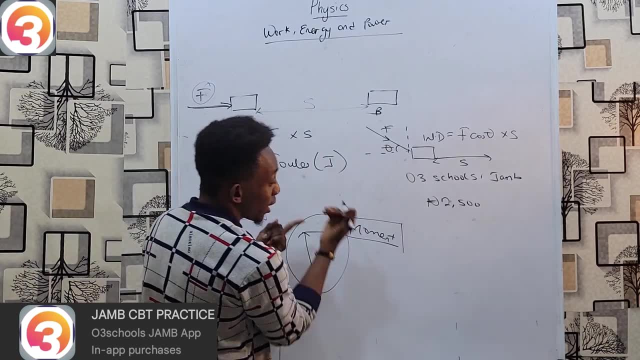 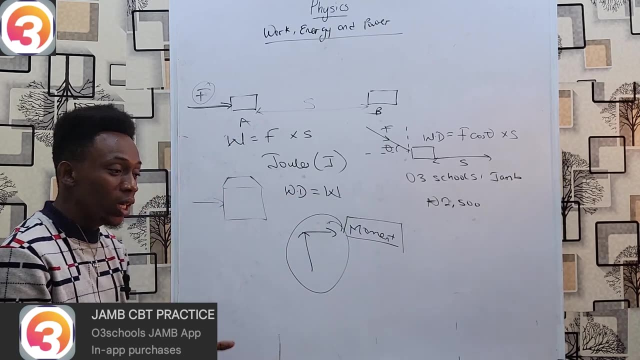 important thing, you must understand the force and the displacement must always be parallel. that means if i also be raising a weight off the ground and if i'm taking it vertically upwards, then the force i'll be looking at in that case must be the weight, because you need to have high force because of the 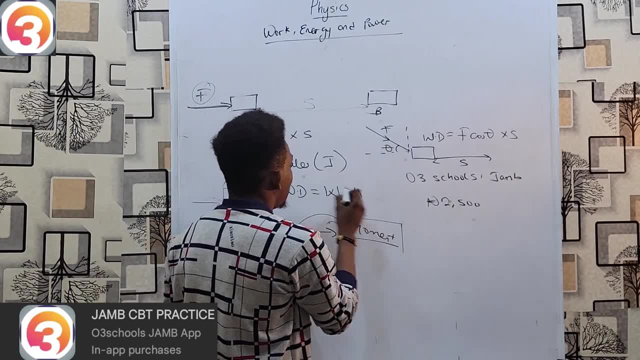 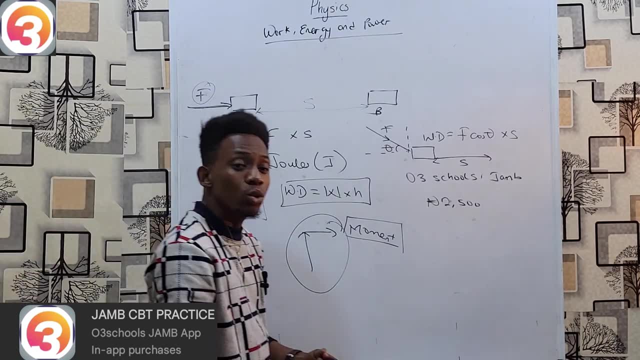 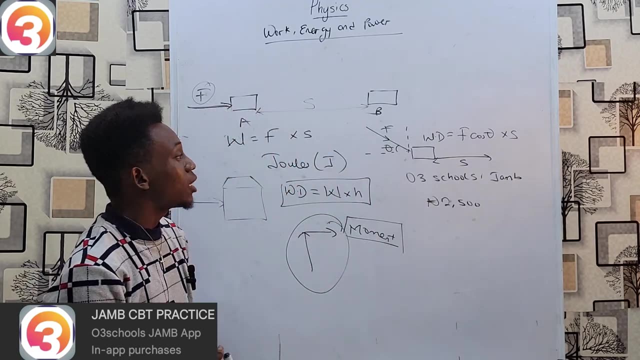 width of an object, to raise it, so that becomes weight times height. and that is what you must know if i work. and now move on to energy. what is energy? energy is the ability or the capacity to do work. that means, while moving these objects, these distances by applying force, the thing that 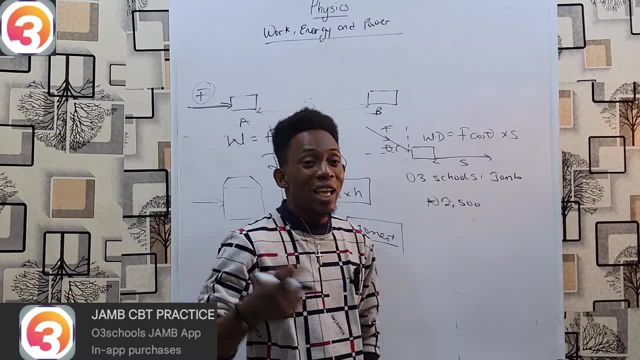 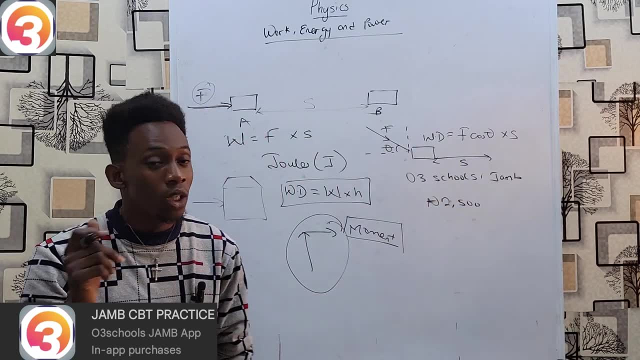 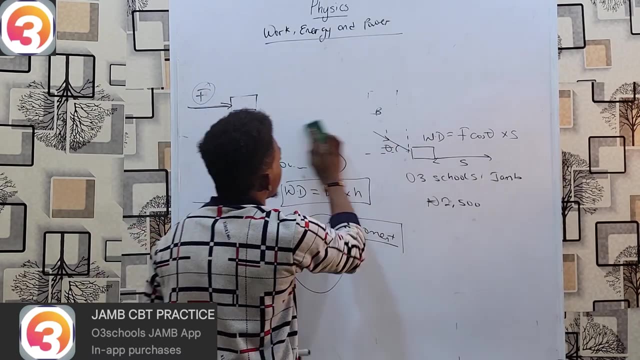 gives us the ability to do that in the first place is now energy. now there are so many types of energy, and so our way of generating energy- now this is- are very complex in energy space, as well as the amount of energy going back and forth. there i can easily root a particular type of energy. 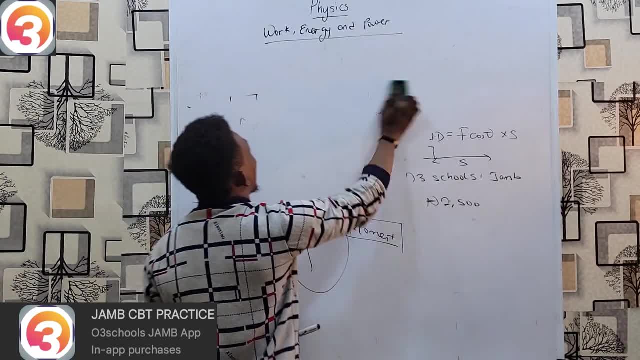 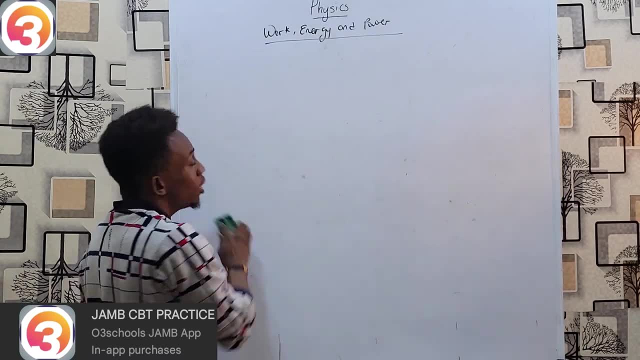 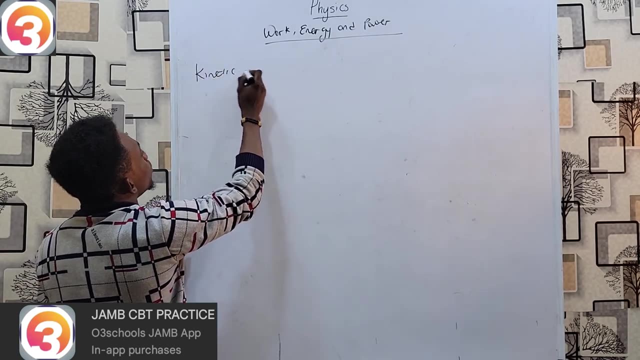 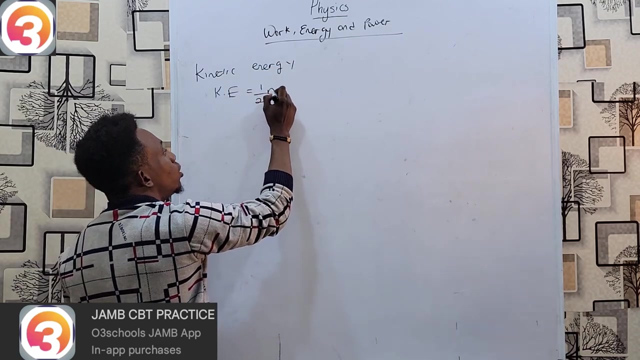 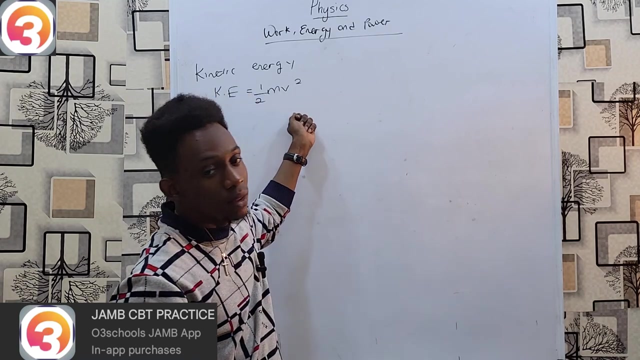 between these other different types of forms. the first thing is the open space. you see, with the open space you have potential energy, kinetic energy and so on. form my, a moving body, and its formula simply becomes one over two: mv squared, half mv squared one by two times the mass and the square velocity. that is kinetic energy. now, on the other hand, potential, 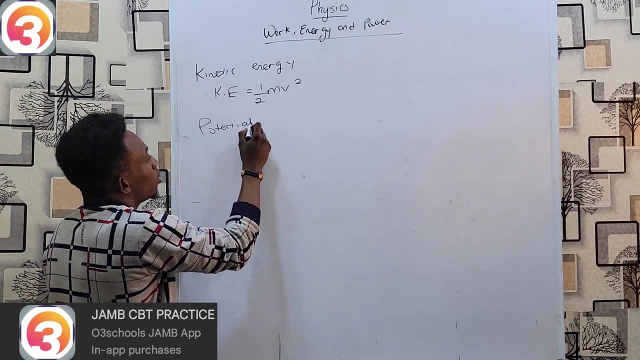 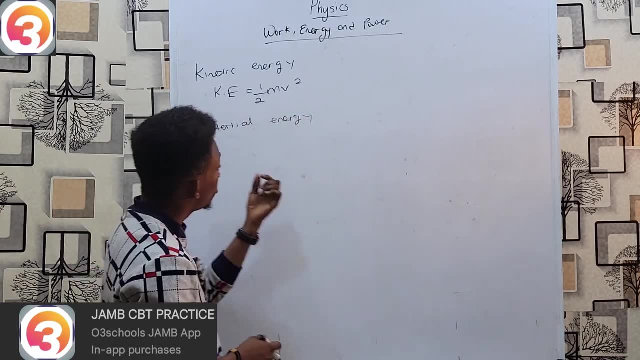 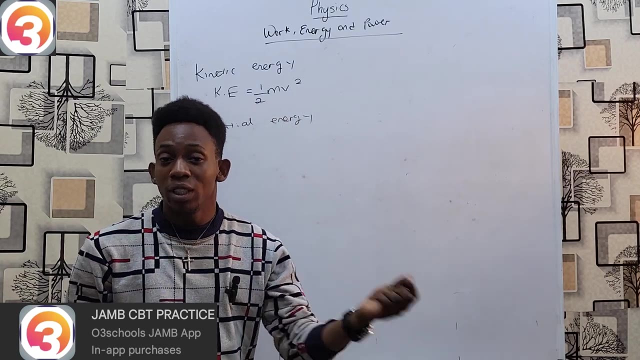 energy is the energy possessed by a body by virtue of its arrangements, position or states. one more time: position energy, energy possessed by a body by virtue of its arrangement, position or state, and they are cemented as a potential energy. there is your chemical potential energy, there is. 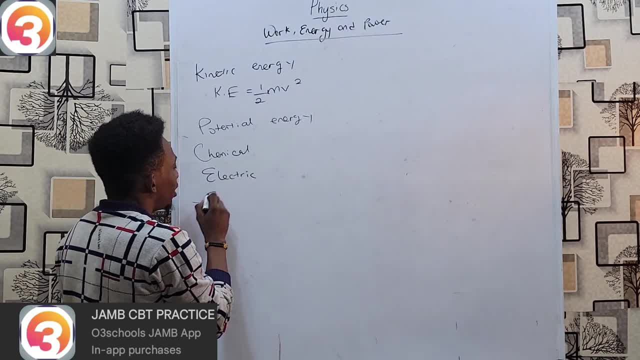 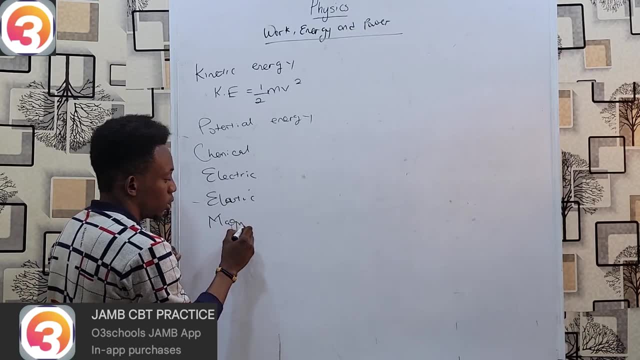 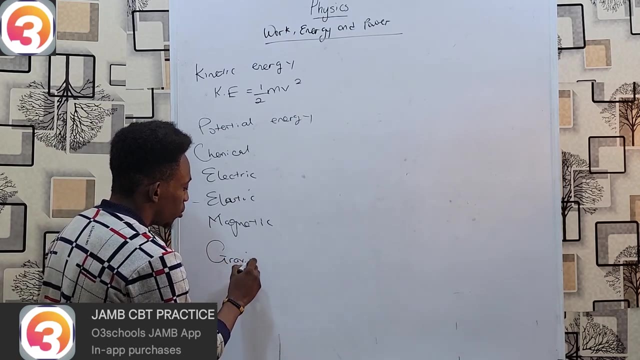 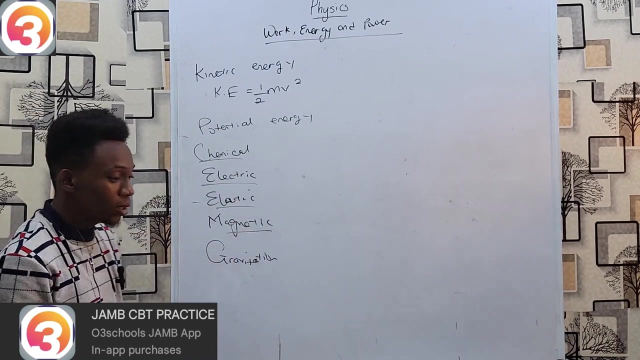 electric potential energy. there is elastic potential energy. there is- uh, your magnetic potential energy, but right now we are going to be focusing on just one of them, which is the gravity of the body potential energy. the rest of these are all stored individually under different topics. the only one, 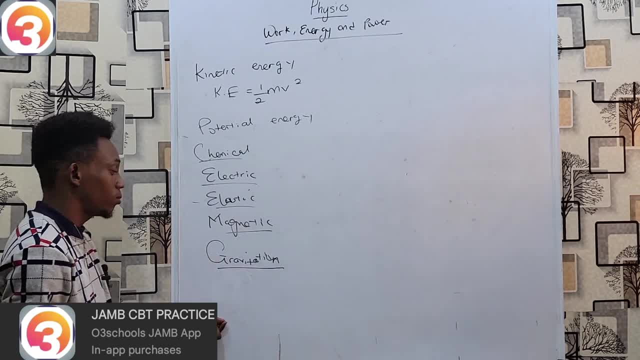 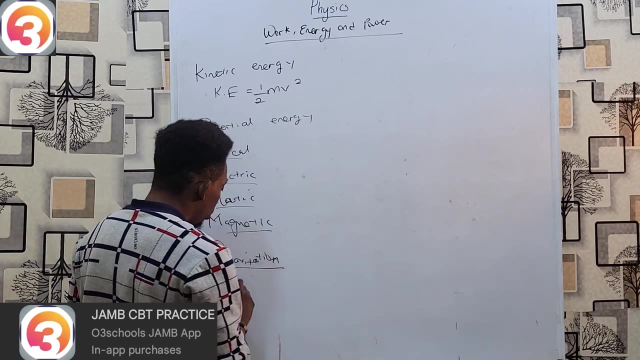 we're focusing on right now is your gravitational potential energy, and that's the energy being possessed by a body by virtue of its height above the ground. you raise the stone up. if you drop it, the stone has gained energy. that energy is fatal, as gravitational potential energy and its formula 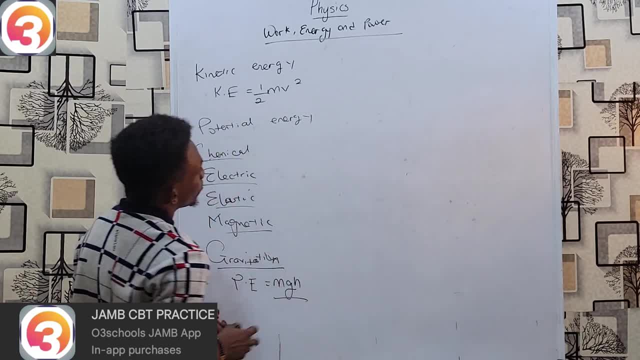 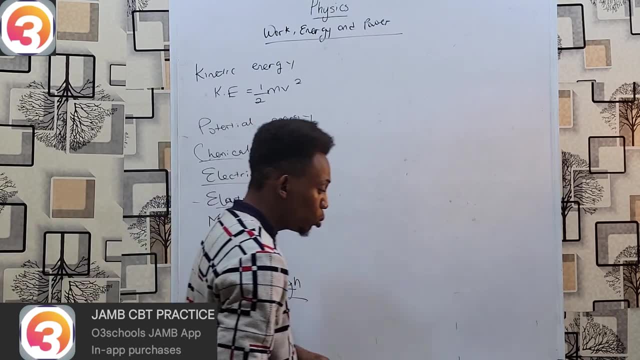 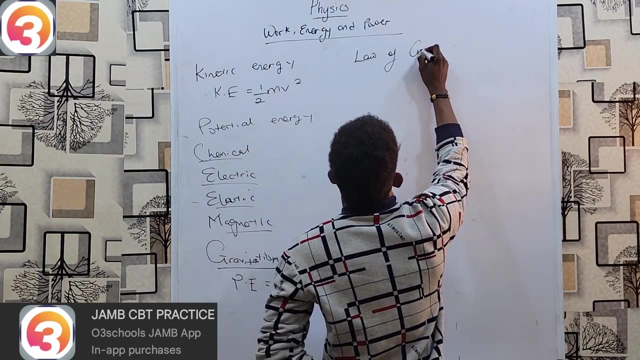 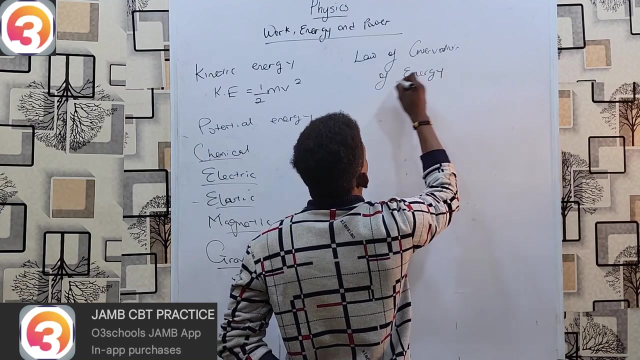 is um, g, h, mass times, acceleration to gravity times, height. and now this leads us to one of the most important concepts in physics, which is the law of conservation of energy. and this law is quite simple: it states that energy can neither be created nor destroyed, but can only be transformed from one. 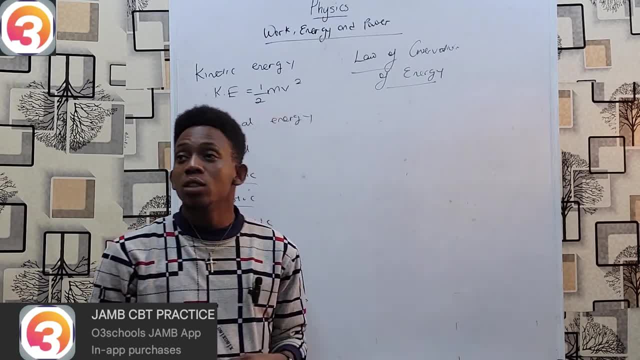 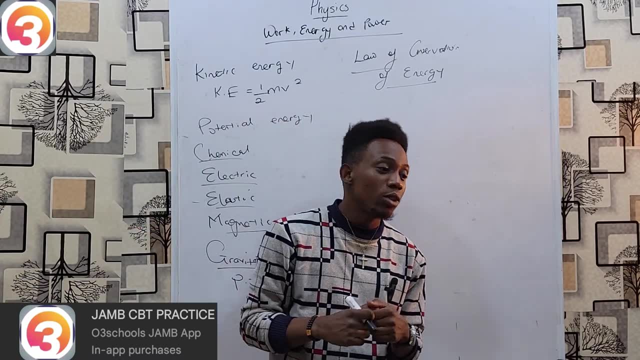 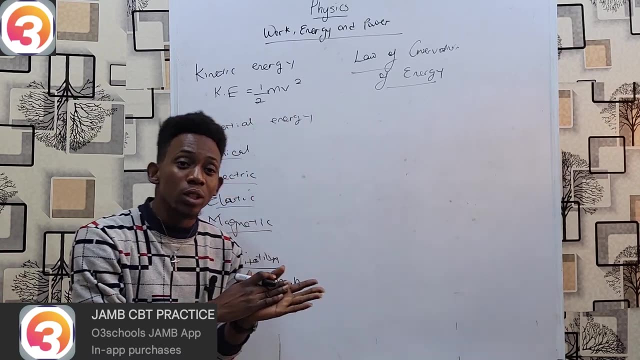 form to another. that simply means that the sum of all the energy in a system remains constant. the energy is not going anywhere, it's not being created from nothing and it's not being destroyed. it's nothing either. it is simply transforming from one appearance to another. say calm, say, for example, you have to iron. 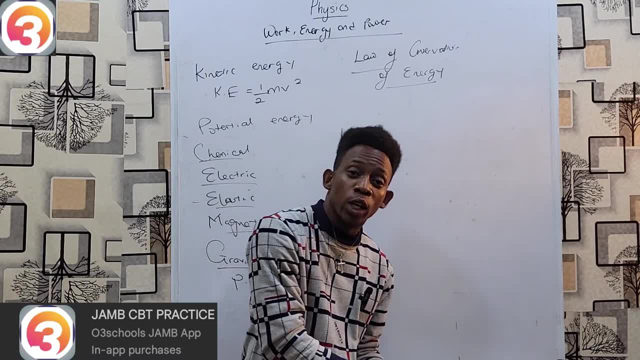 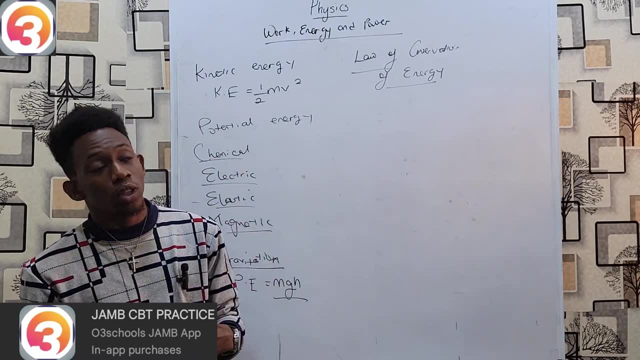 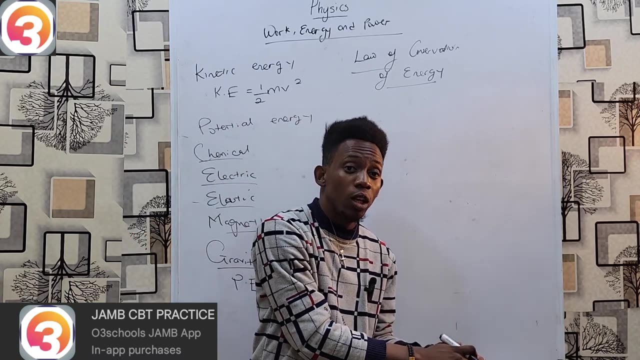 your clothes, you plug in your iron, taking electrical energy. that energy doesn't get wasted, here's transforming to thermal energy, heat, which you then you suppress your particles, or you want to switch in your generator. for example, you put in foil, chemical energy, switching on this foil makes your doing work and you now have electrical energy. the electrical 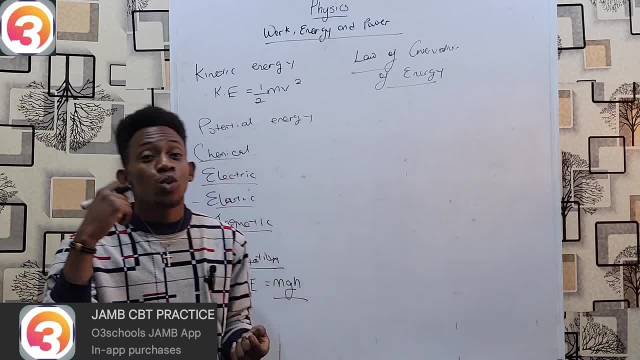 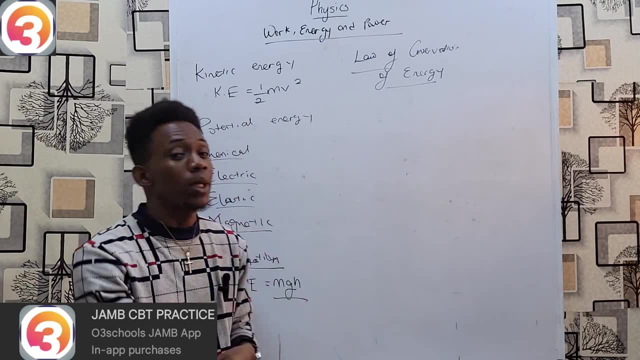 energy could be transformed to your fan, for example, to give you kinetic energy, to be transferred to your bulb to give you light energy, to your heater to give you thermal energy. you can all see now, the important principle about this law is that if you have to start with 100 joules of 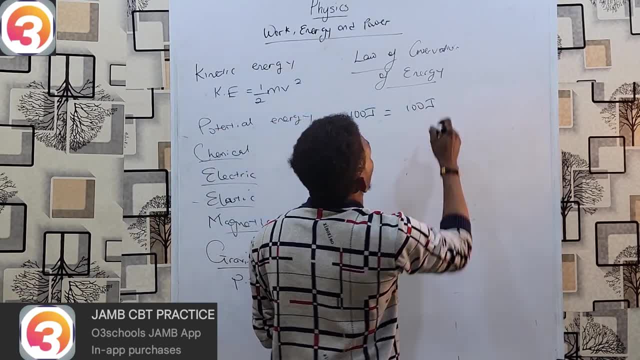 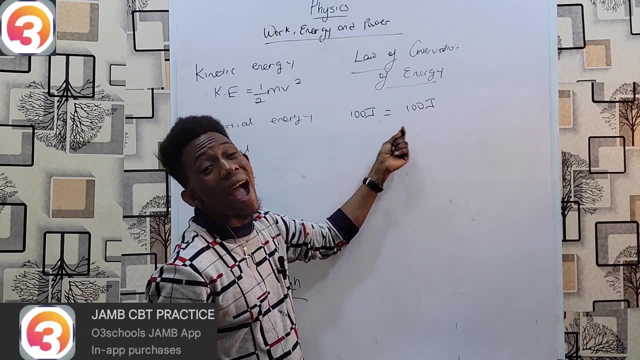 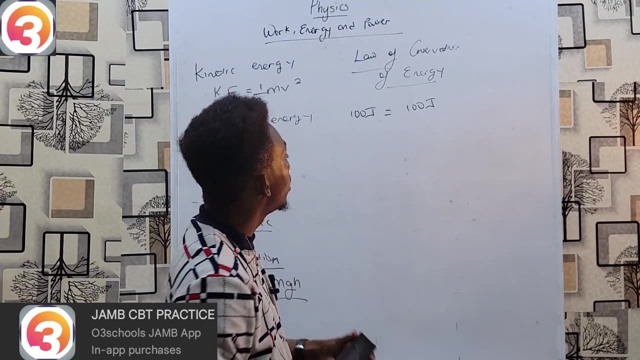 energy. you should also be ending up with 100 joules of energy, albeit in a different form, so you should say 100 joules. it just might no longer be how it's factored initially. that's the basic thing. now, a good example or a good way to analyze this is to think about a stone being dropped to. 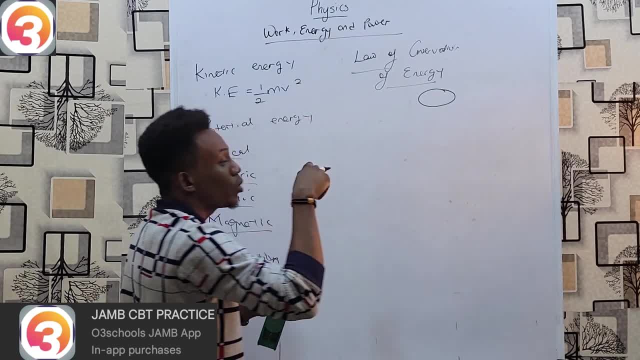 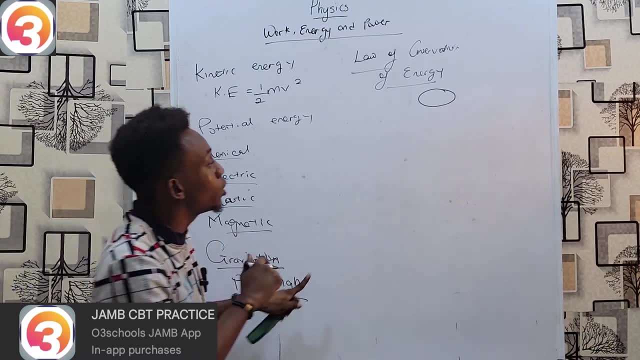 a certain height. now, once the stone has been raised up, you remember, you notice that has gravitational potential, energy, because you will notice that the energy will be coming out from the of its height above the ground. and why i'm holding this stone at this height, all it has potential. 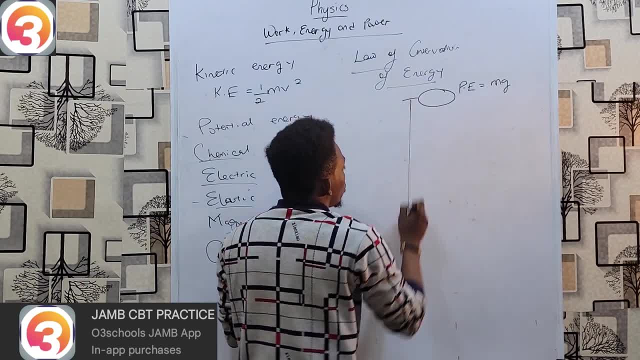 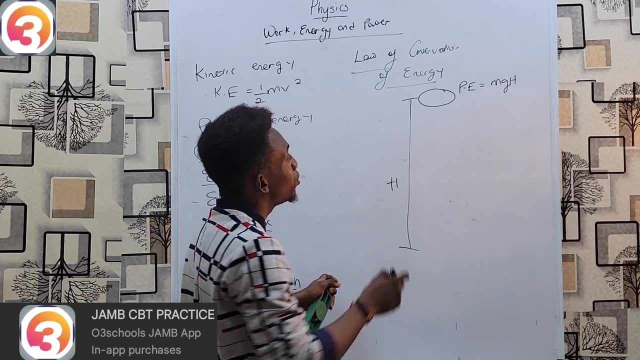 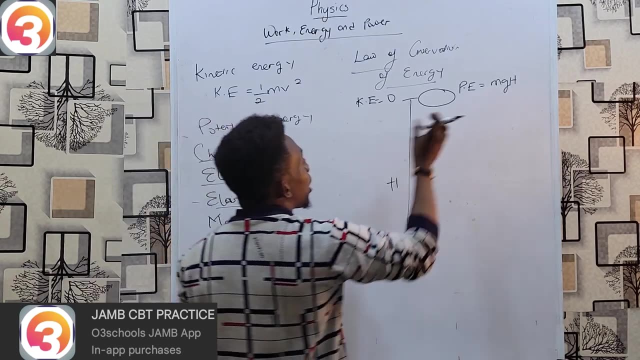 energy, mg, and let's say this is the distance to the ground. i've written h. that's what it has, and because i'm holding it at that height it is not moving. its kinetic energy must be zero because velocity is zero. you see, this is now the maximum energy. now say i leave the stone, it begins to fall. 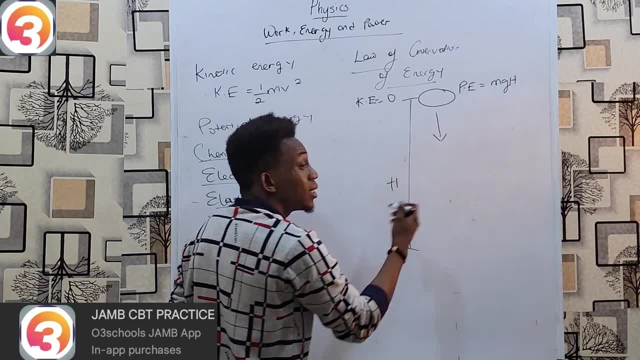 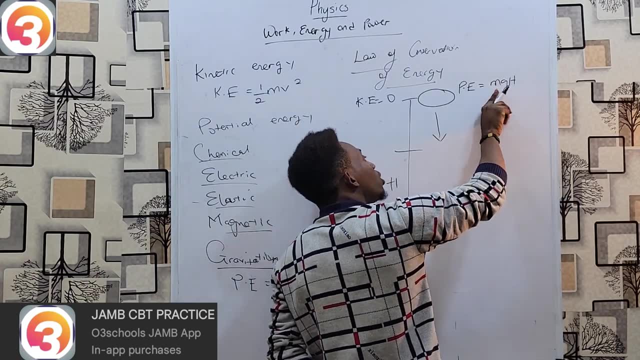 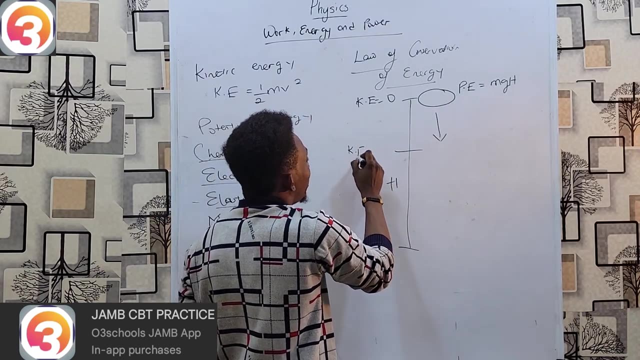 as it falls, its speed is increasing and increasing and increasing. so at a certain point here the potential energy would have reduced from what this value was before to a new value. however, the kinetic energy would have gained every single part of the potential energy that got lost. that means 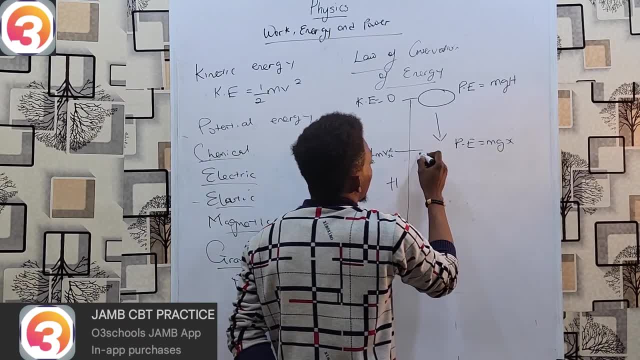 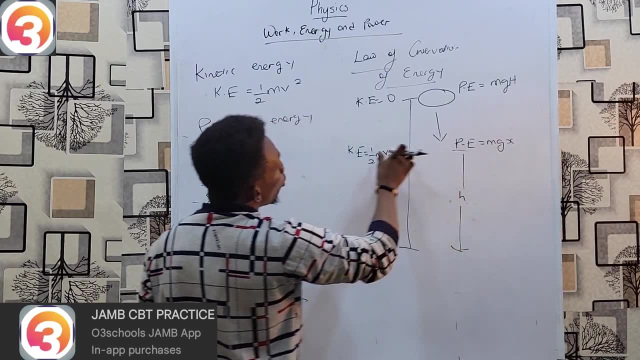 as you are losing part of your energy. the energy is not going nowhere. it's simply been transformed into a different form of energy. the potential energy gets transformed into kinetic energy and as this potential energy keeps on coming down, it's reducing, it's reducing and it's reducing. 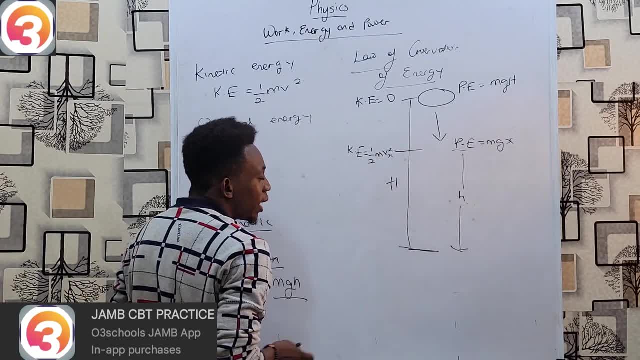 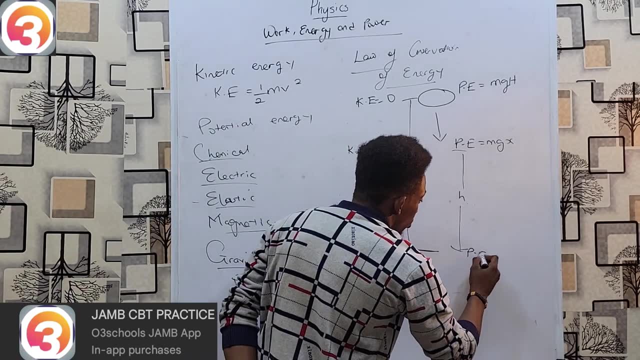 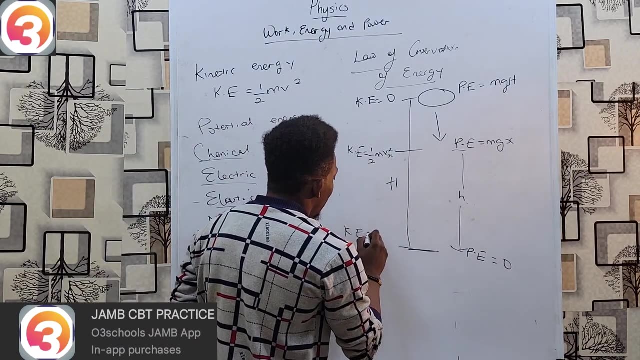 then, at this point, right as it's about to hit the ground, its distance from the ground becomes zero and, as you are aware, mg times zero must give me what zero. the initial energy gets here and reduces to a null value. it's now zero, oh. the kinetic energy, on the other hand, now reaches 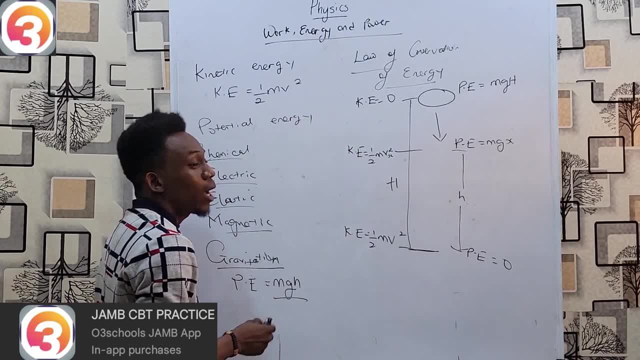 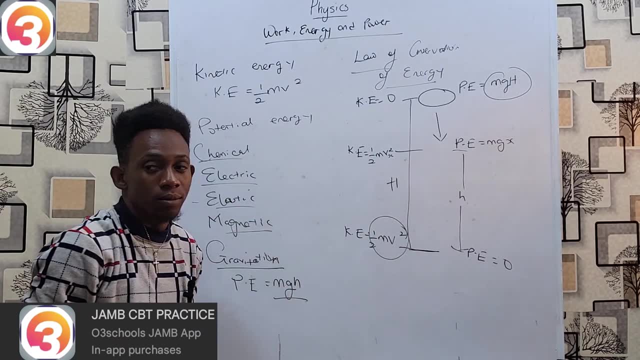 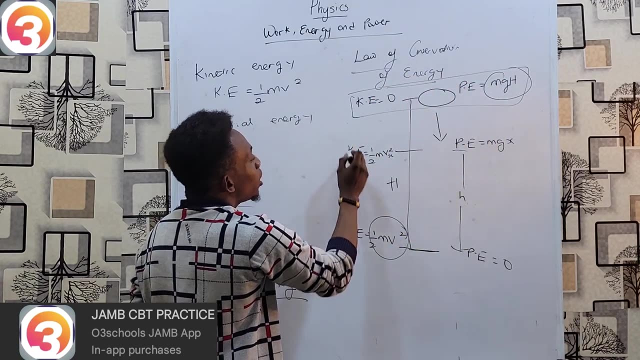 the maximum value that means at this point. all this potential energy has now been converted into purely kinetic energy, but the important principle to remember is that the total energy we have here will still be equal to the total energy we have here, and they can still be equal. 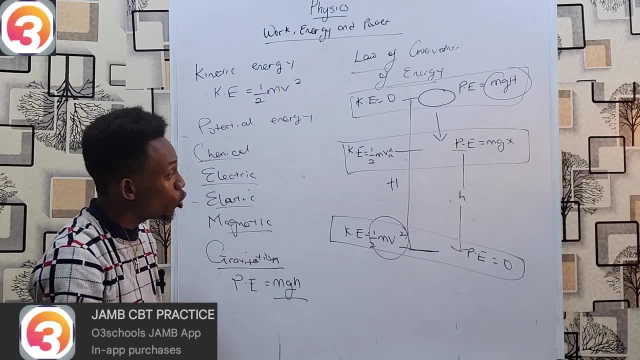 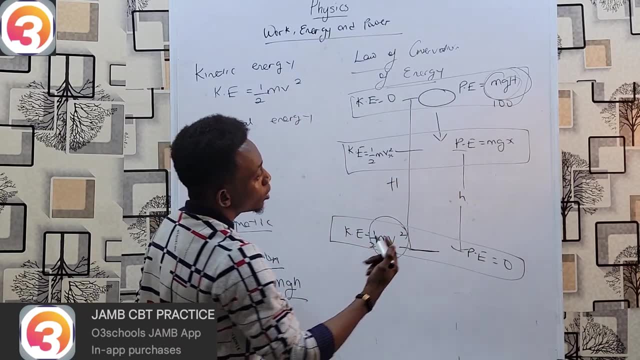 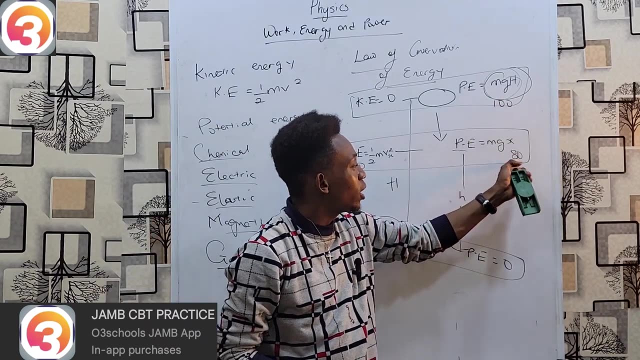 to the total energy we have here. energy doesn't go missing potential energy, as it's reducing. it's reducing if this was 100 years, as it's reducing if it gets to 80. this guy must now become 20.. the 20 it has lost between 180 gets transformed into kinetic, and so, as this kinetic keeps on, 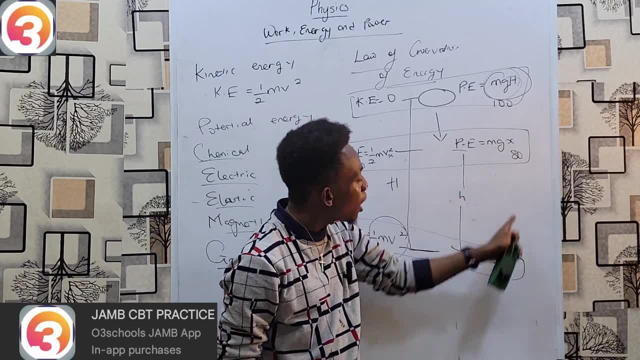 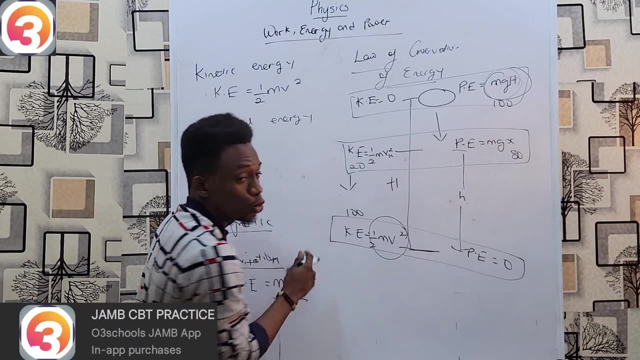 increasing, but it keeps on reducing until the potential becomes zero one more time, while kinetic would have gained every single thing and now become 100.. so that's a very simple and accurate example of how the love of kinetic energy has changed over the years. so that's a very simple and accurate example of how the love of kinetic energy has changed over the years. 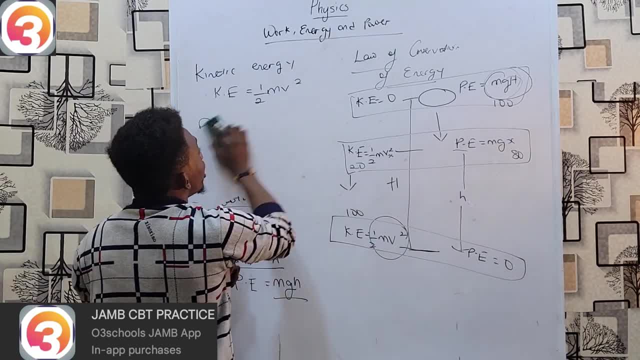 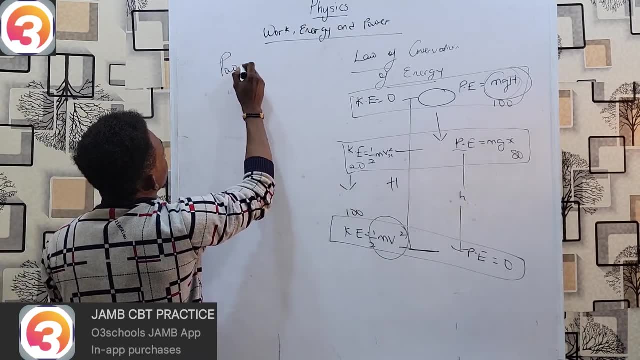 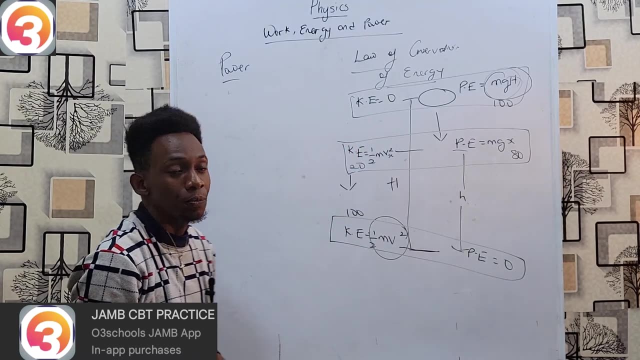 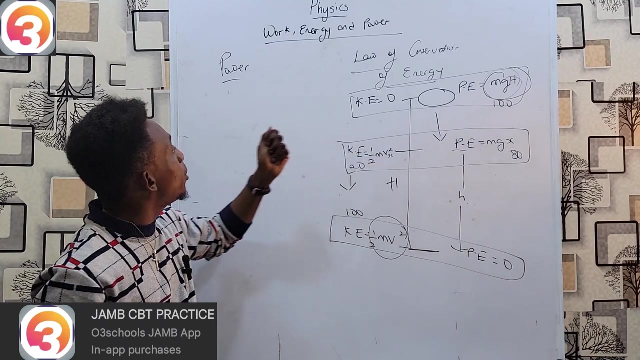 is applied and once we know that, you can then look at the last important concept, which is power. power simply refers to the rate of doing work, how fast you can perform your work. the faster you do your work, the more power you are said to have. our energy and work are measured in jews. power, however, is measured in a totally 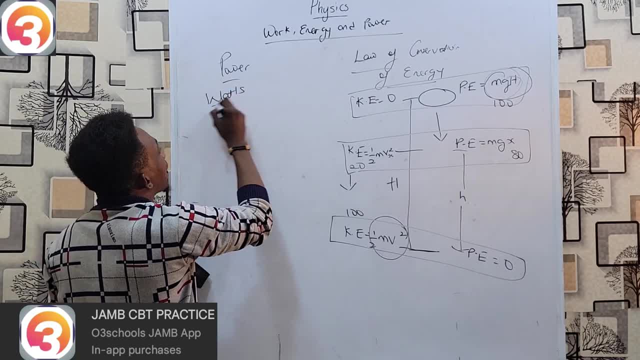 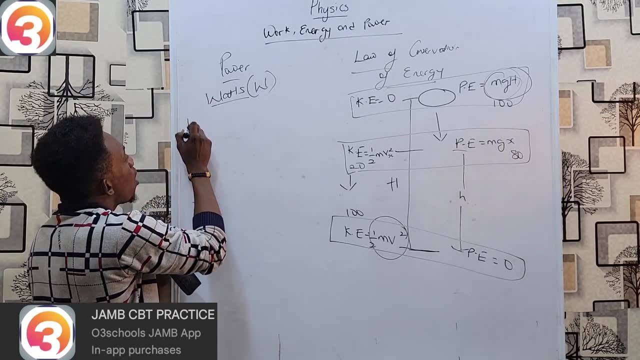 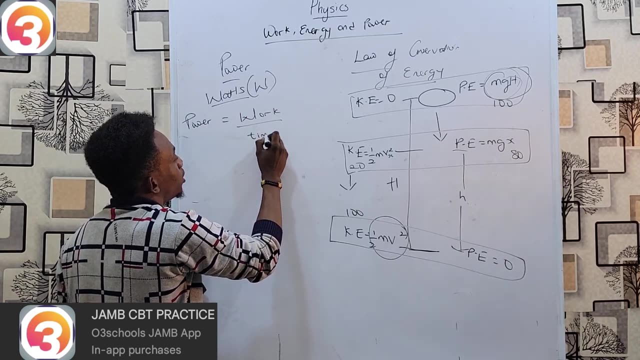 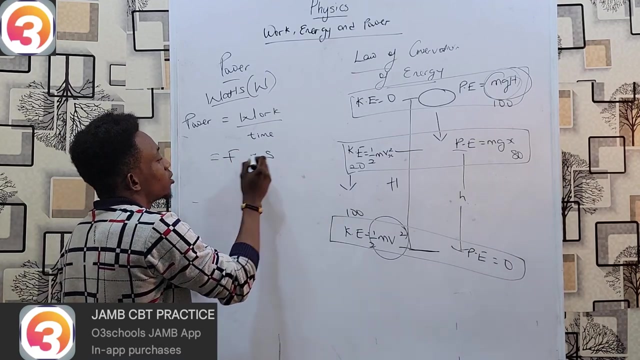 new unit, which is watts or calculator w. power is measured in watts and the formula for power is going to simply be work, or energy, simply divided by time, work over time. and, if you remember, work is force, times, distance. so, over time, oh, three-month primary school, which you should still remember, we're all. 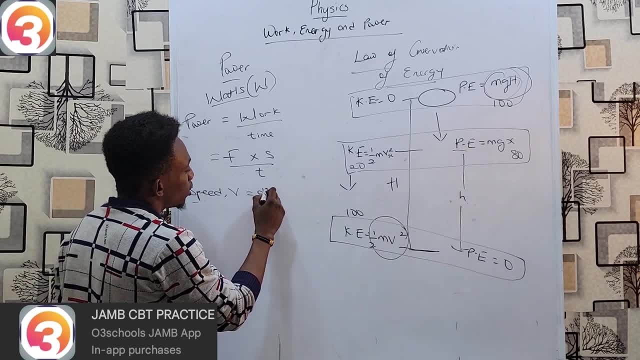 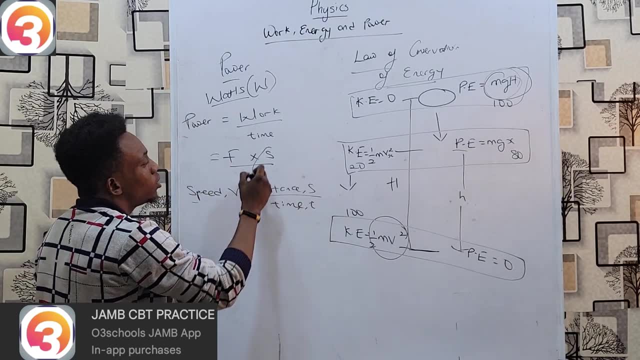 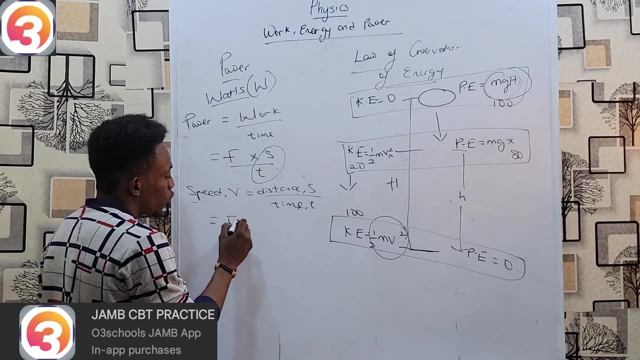 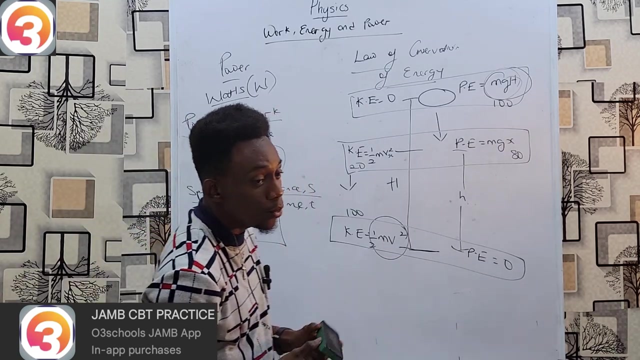 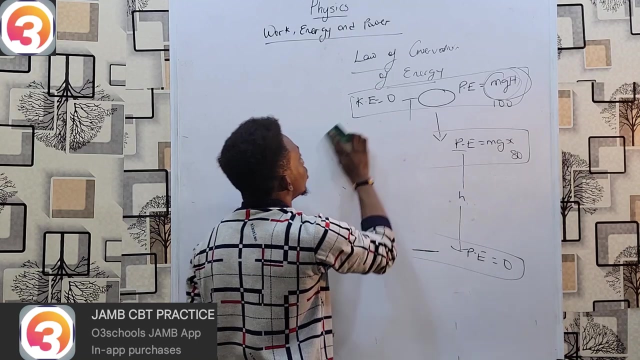 always knew back then that speed equals to distance over time. that means this particular guy there alone represents speed or velocity, which means that powers be equals to force, times, velocity, and with these i believe we are ready now to assess. uh, all three schools jump up and take some past questions to further enhance our understanding of the topic. so let's do that so. 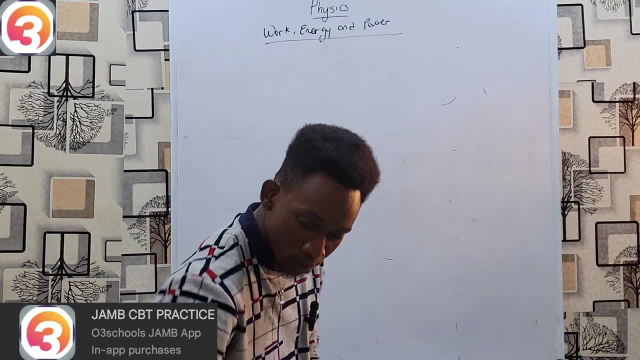 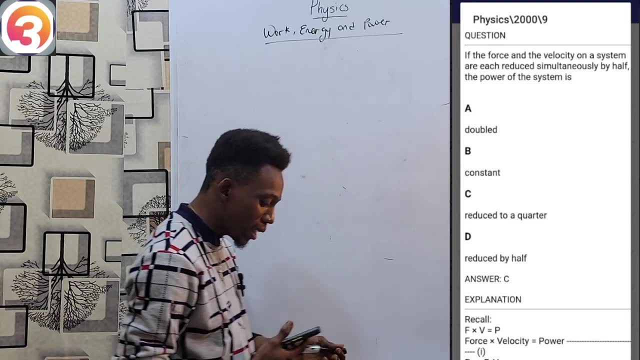 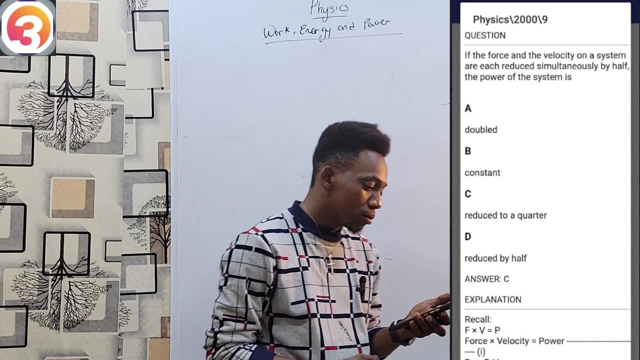 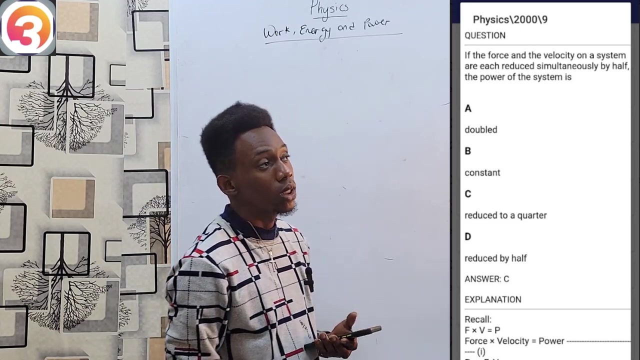 setting through your past question by topic, like i said you can do. you can start with um 2000, question number nine, the year 2000, question number nine. this question states: if the force and the velocity on a system are each reduced simultaneously by half, the power of the system is what that means. if, say, the force was f and velocity was v. 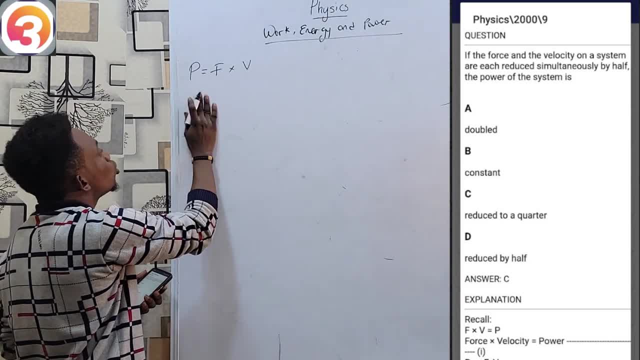 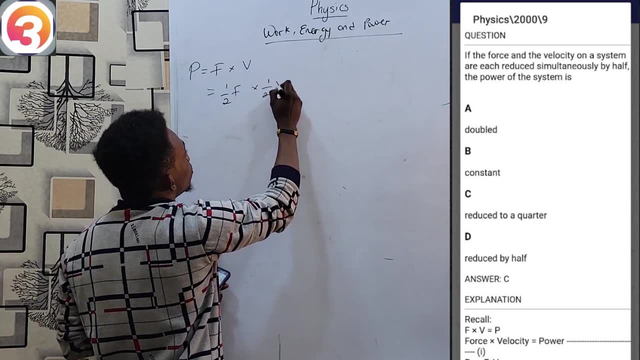 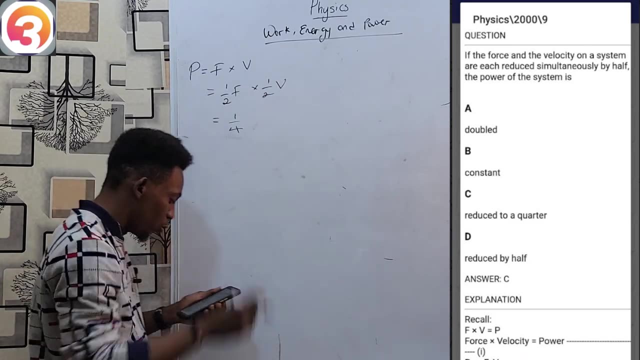 this p will be our power. then if we were to reduce the force by half, we can need one over two f, and also the velocity by half, one over two v. what happens to the power? one times one, one, two times two, four, that means our power is 1 over 2v. 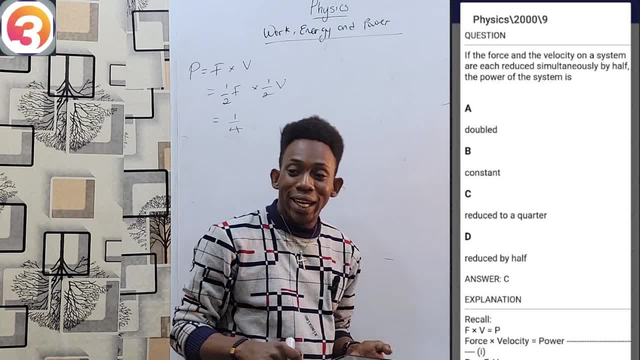 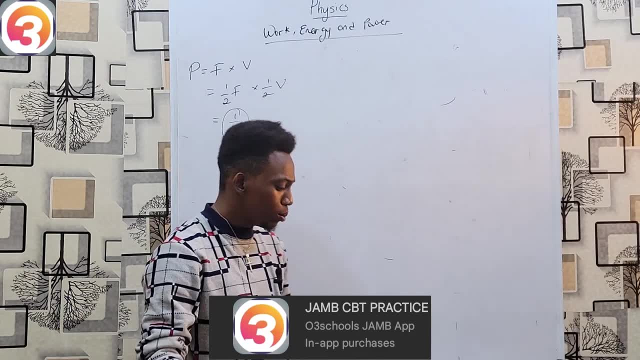 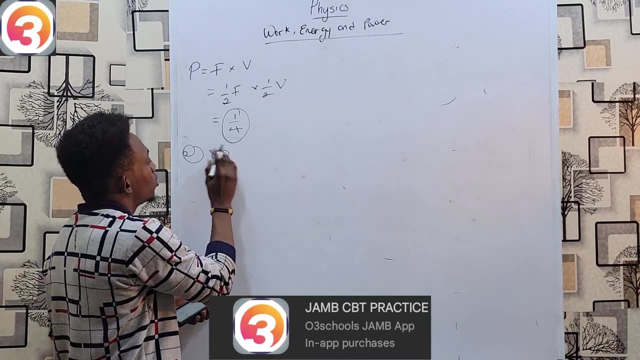 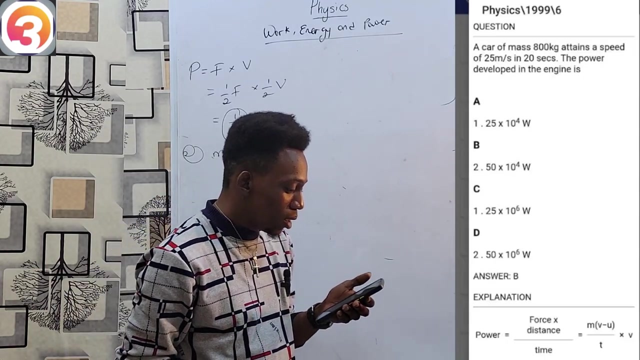 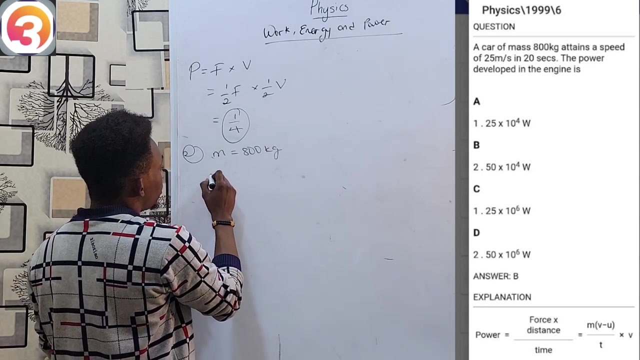 that means is reduced to a quarter. 1 over 4 is a quarter, and that's that. see, is that simple. for our second example: a car of mass 800 kilograms. a car of mass 800 kilograms attains a speed of 25 meters per second. speed of 25 meters per seconds. 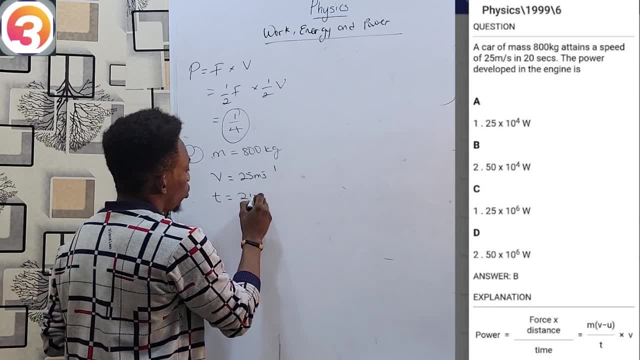 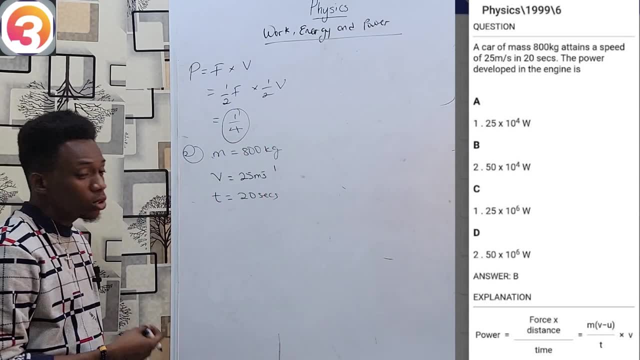 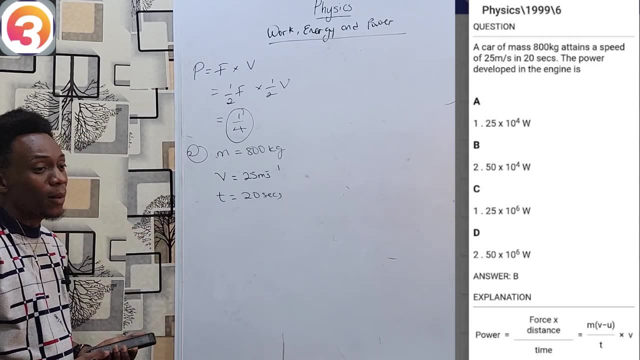 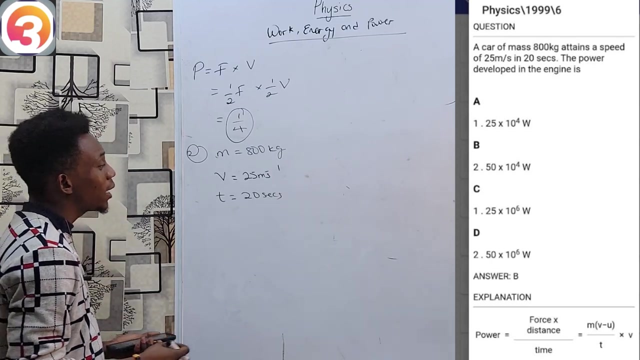 in 20 seconds. the time is 20 seconds. we have to find the power being developed in the engine. now this question might seem a bit tricky because you remember that power should be four times. then you simply have to ask yourself: all right, what can i do? can i find how far this vehicle? 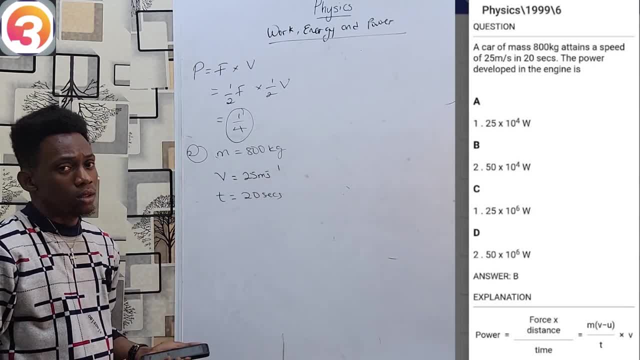 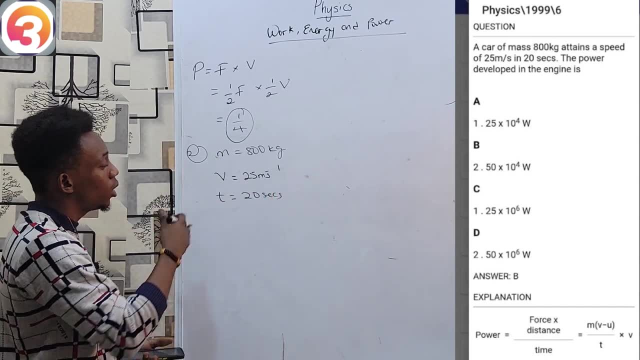 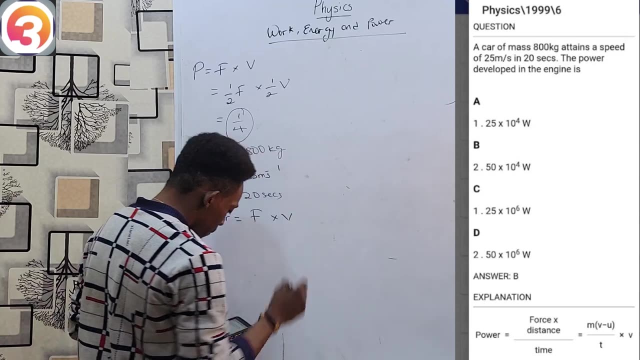 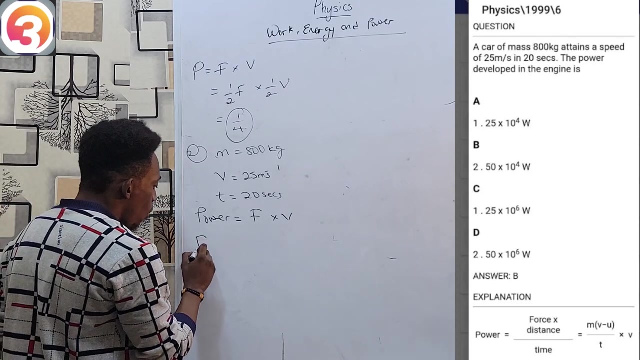 would have moved in this interval. you see how we reason it out. take from what you do and try to walk towards what you want. i want to get power and then the power is force times velocity. so i might know velocity promises to get force, then remember force equals mass times. 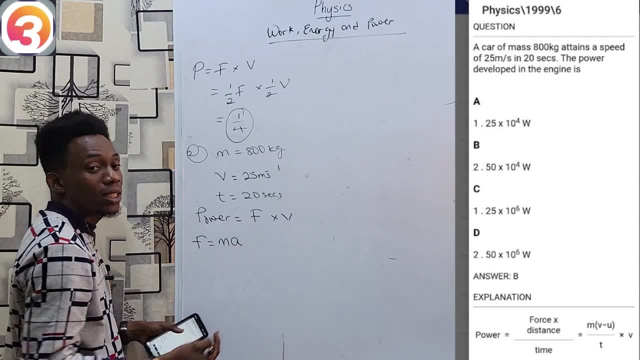 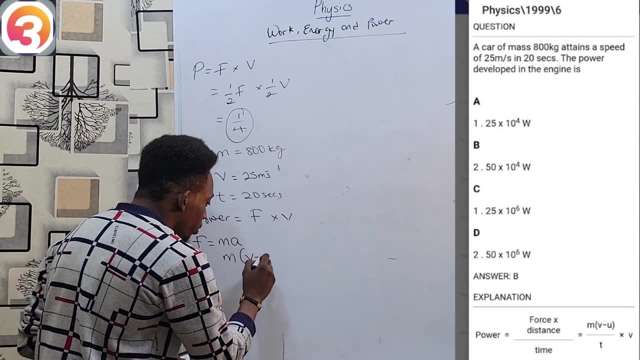 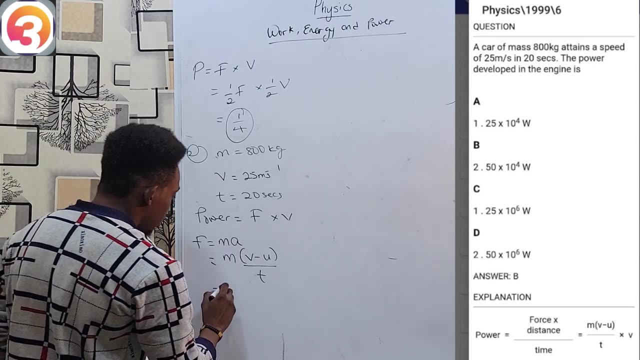 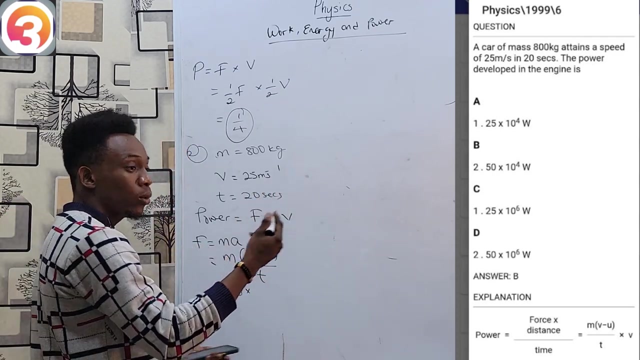 acceleration. that means if i can get my acceleration, i can get my force. how you might? acceleration solution is changing velocity over time. see. so, quite simply, my mass is 800 and my acceleration is over. add yep, so uh, this means 식. my change velocity is that this car is moved from 0 to 25, so 25 minus 0. 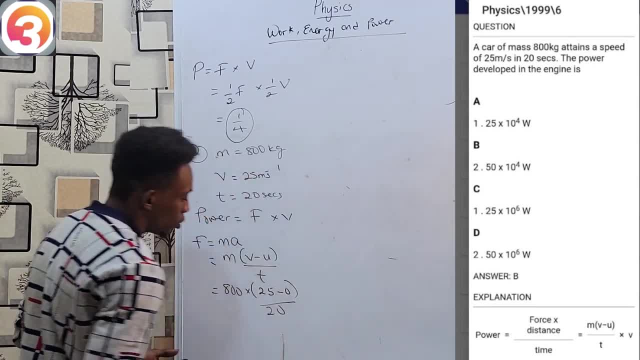 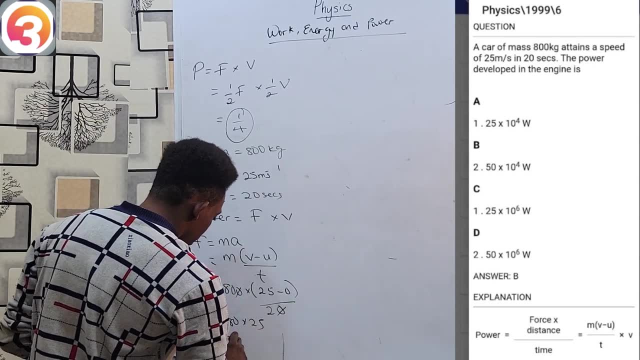 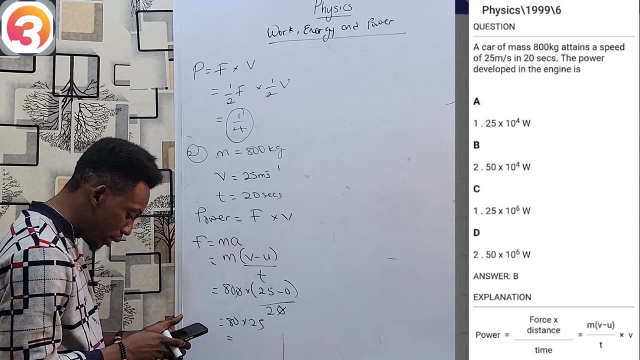 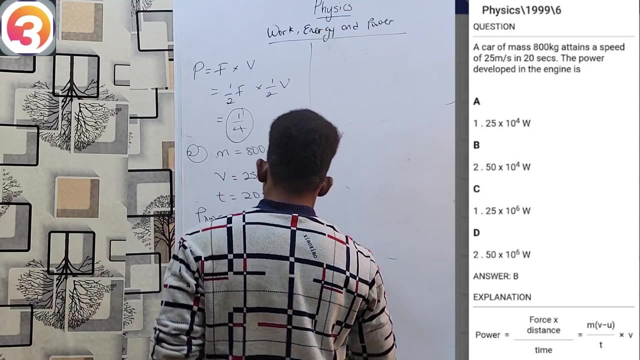 all over the time, which is 20 seconds, and so we know that zero can cancel zero. that is now with 80 times 25, and if you press that into your calculator, quite simply we know that 80 times 25 is 2 000, so my force is 2 000 newtons and therefore my power must be. 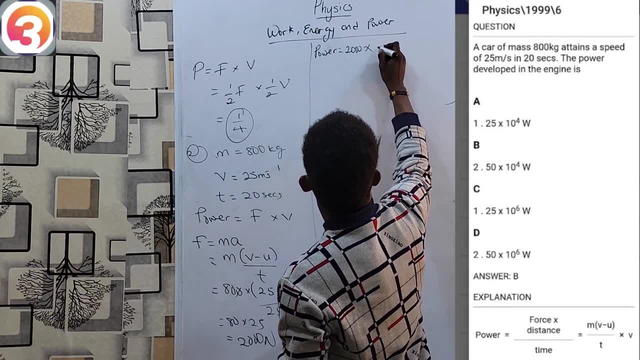 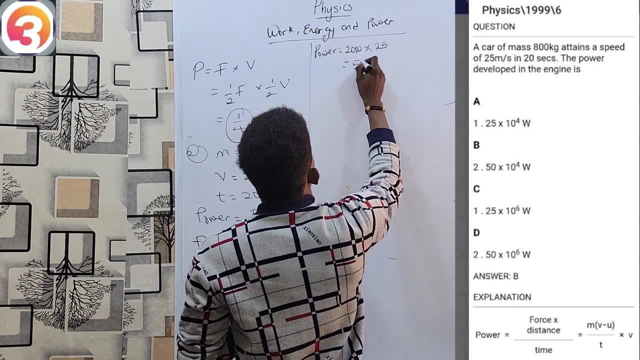 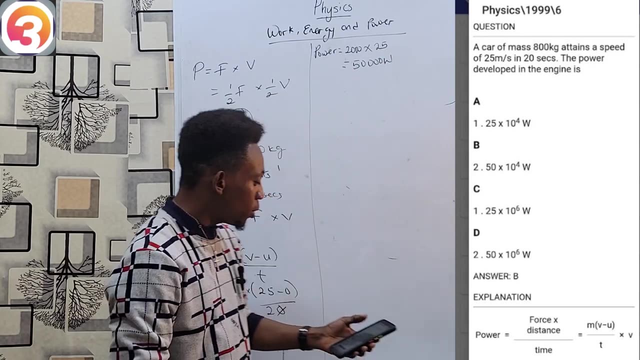 2 000 times the velocity, which is 25. so 2000 times 25 will give you 50 000 watts. and then when you take a look at your options, okay, and now when we take a look at our options, we notice our answer is not quite among the options. 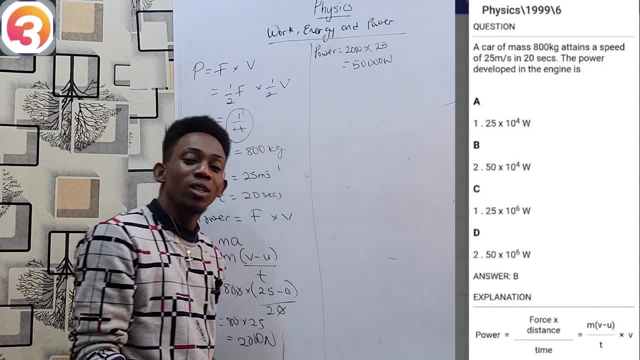 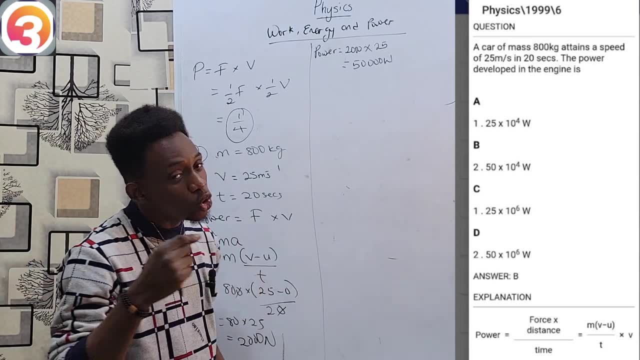 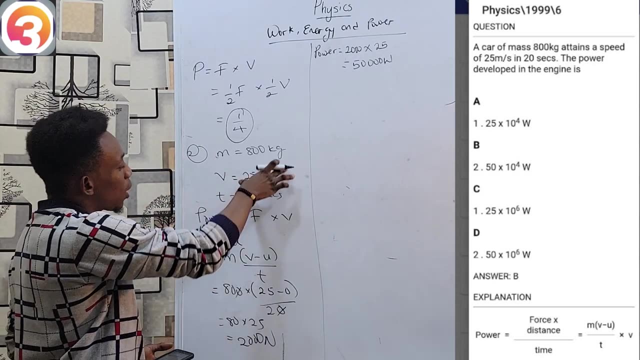 now. this is to remind us that again, we are only humans and mistakes are inevitable. now, a key element in exams is to always be able to spot your mistakes and try and avoid them later on. now, if we go through our questions, we look: here, these are our values. we went through this. i think some of 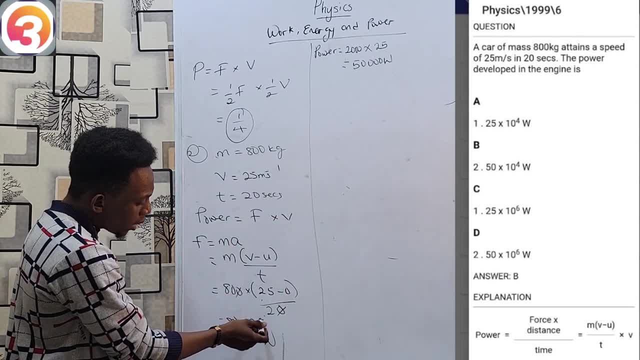 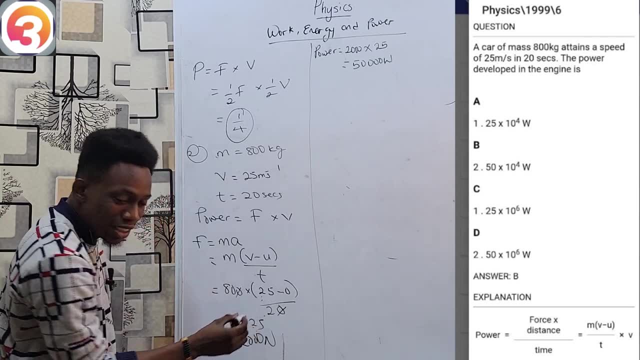 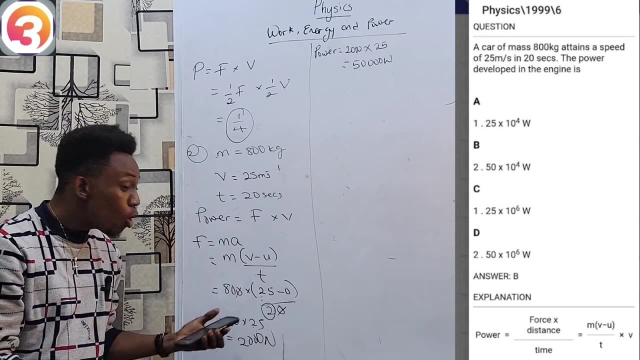 our math and change velocity over time, and here you can notice this must be our mistake, because 25 minus zero is 25, but we seemingly neglected to divide by the time, which is two. you see, so small mistakes like that could lead to your answer not being in your options. that simply. 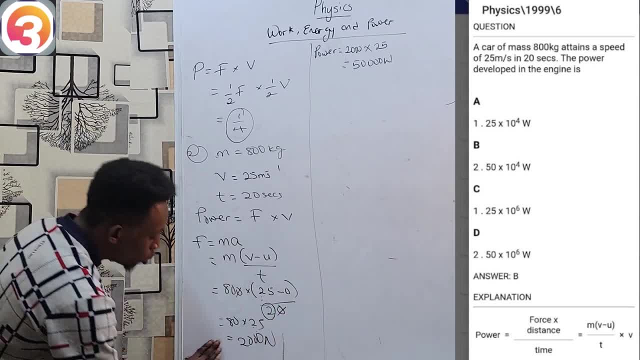 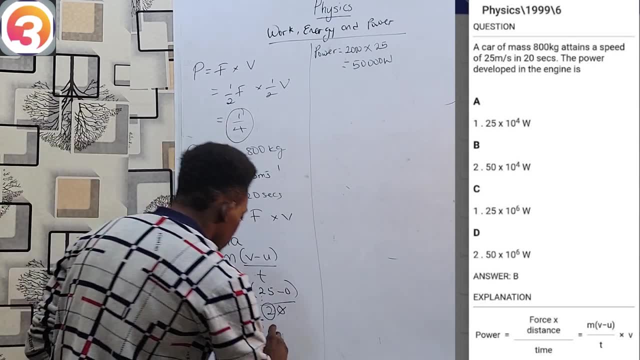 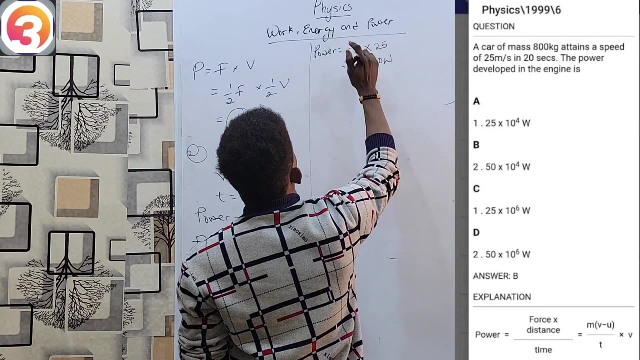 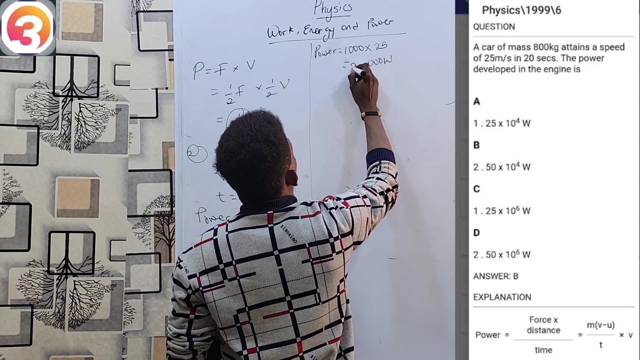 means. our only error was that we did not divide by two, which means this should be 80 times 25, all over two. but we forgot that, and that gives you one thousand newton, and so here, rather than having two thousand, i should be having one thousand. oh, now it's about 25, i'm getting 25 000, and since my options are: 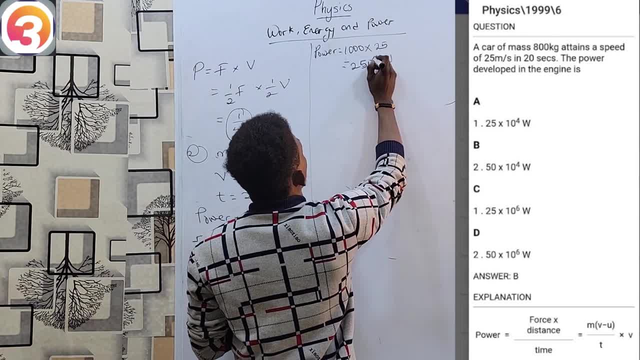 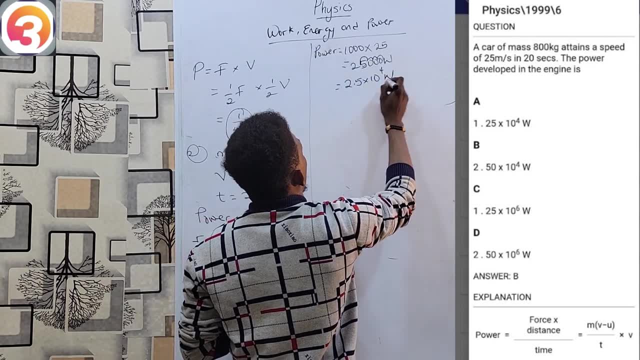 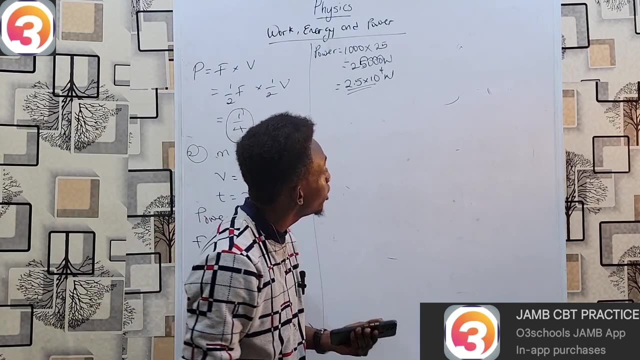 in standard form. if i come back, move back one, two, three, four. i'll be 2.5 times 10 square four, and we see that's how. if you ever find yourself solving and the answer is doing your options, please do not give up and just randomly guess anything number one. instead, try to go through. 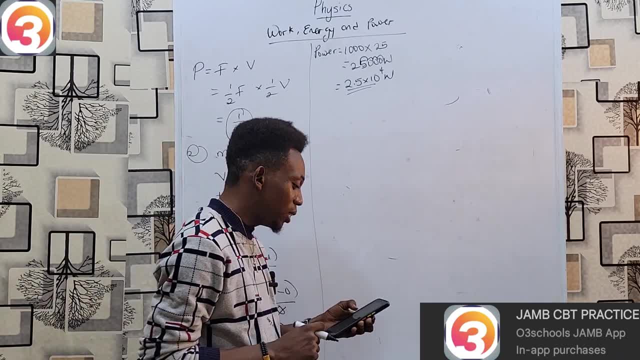 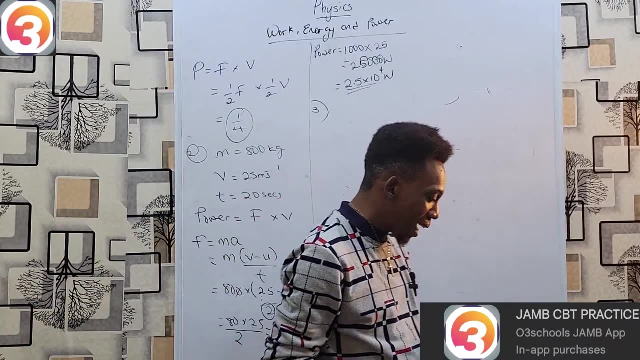 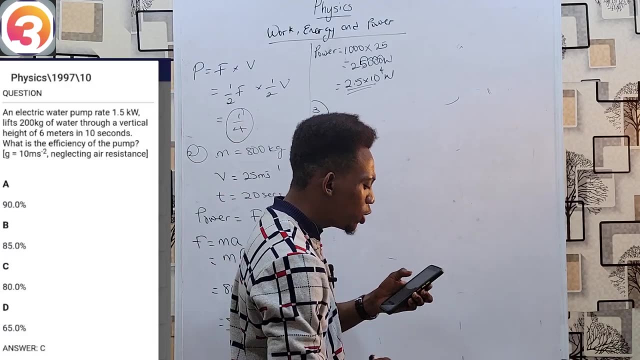 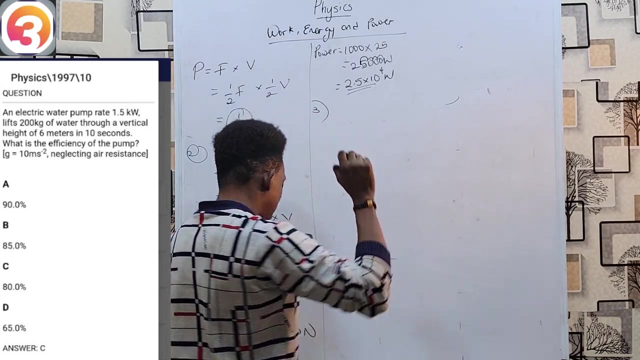 your solutions and see what your error might have been. okay, let's move on to our next question. this question is from 1997, question number 10.. that's 97 question 10.. an electric pump, electric water pump and electric water pumps rate 1.5 kilowatts. 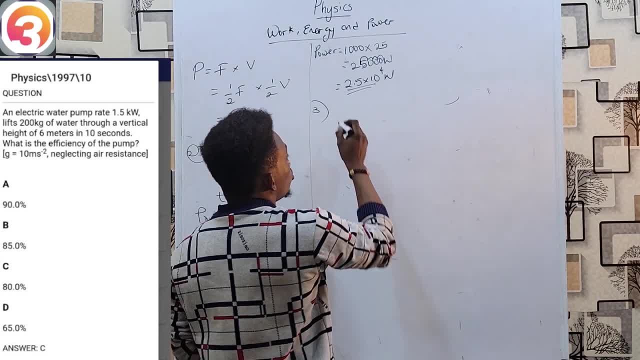 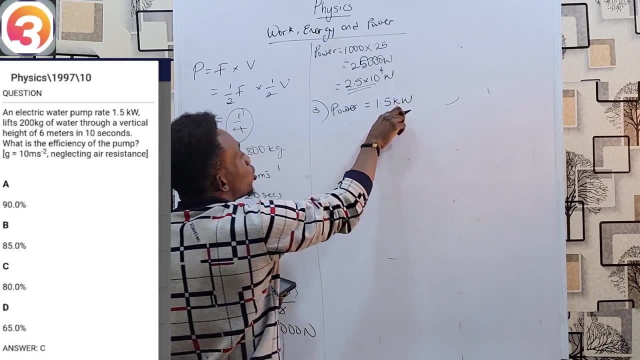 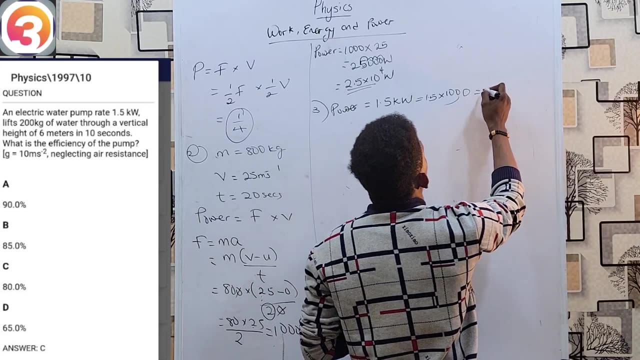 once we hear the rate and we see the unit, that must be our power. the power is 1.5 kilowatts and kill simply means a thousand. let's say 1.5 times 1 000, which give us 1 500 watts. 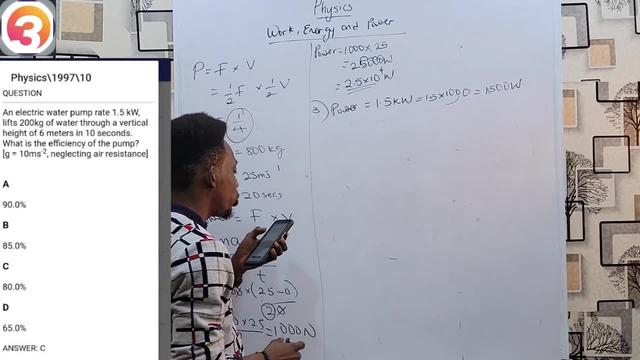 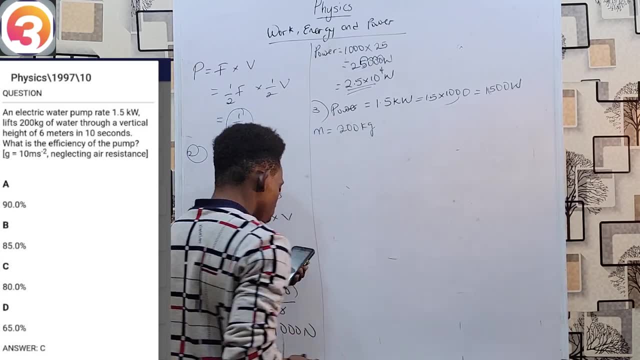 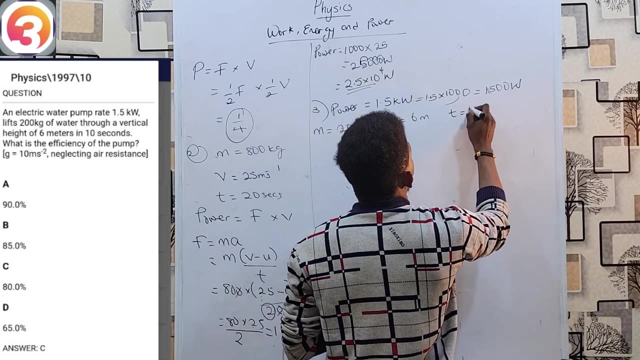 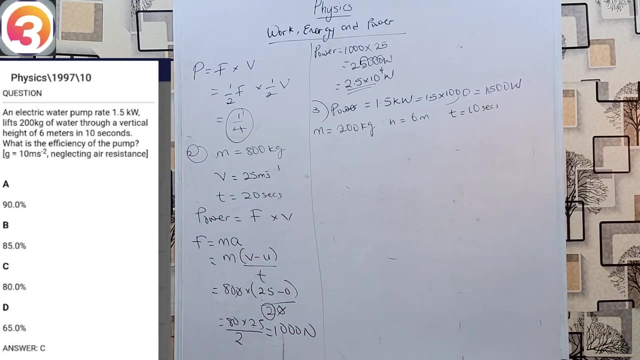 so that's our power and it lifts 200 kg. it's water of mass- 200 kg through a vertical height of 6 meters in 10 seconds. but to find efficiency of the pump, what's going on here? i've been told that this pump has this rate. 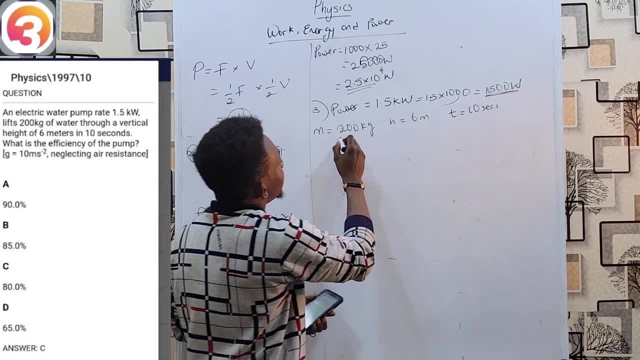 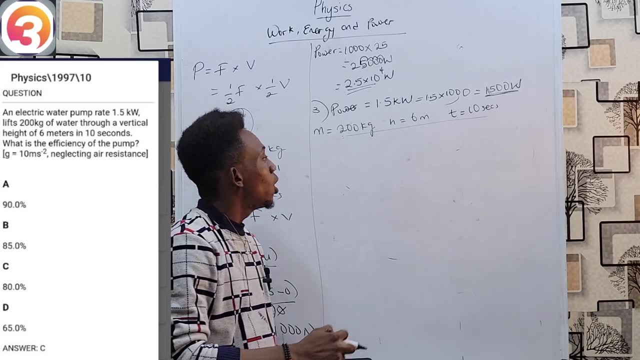 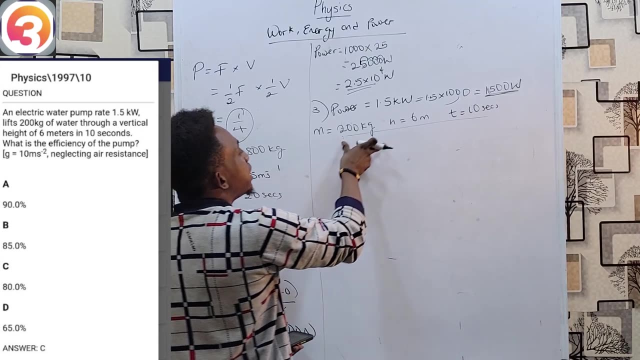 this is the rating of the pump and this is the actual thing it's doing for us, one of the efficiency that is based on what it is supposed to do. how much is it actually performing out of its innate abilities? and first of all, i must solve for the real power that i'm experiencing. and now to solve. 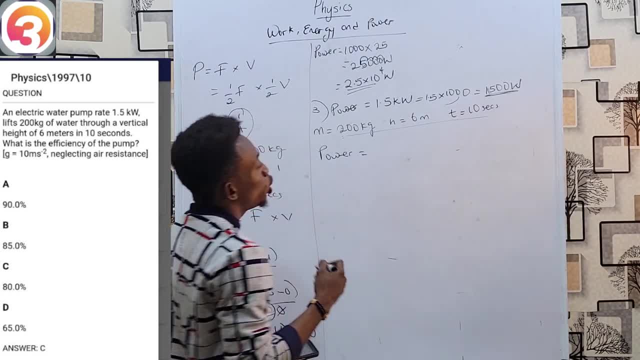 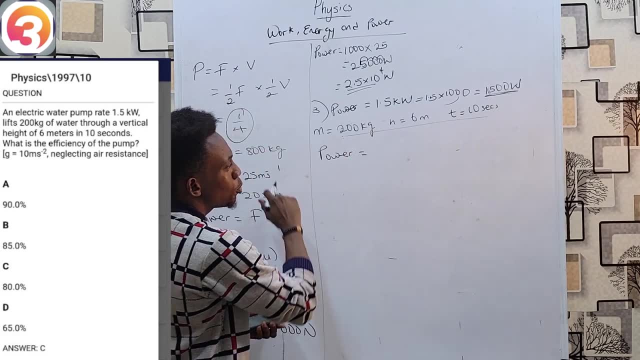 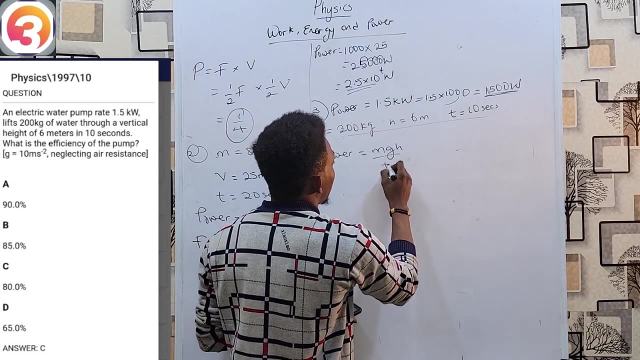 for power. i'll just remember: power equals to work or energy over time. notice, i don't have any stages to solve for work here. but can i solve for energy? yes, let's just go for the work. you're working for potential energy. we are raising this water tray height, so that's mgh over time, so m is 200. 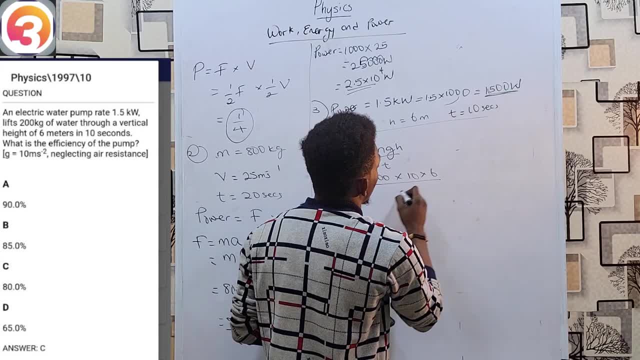 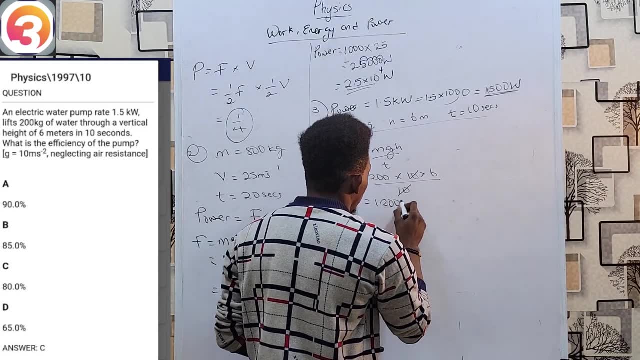 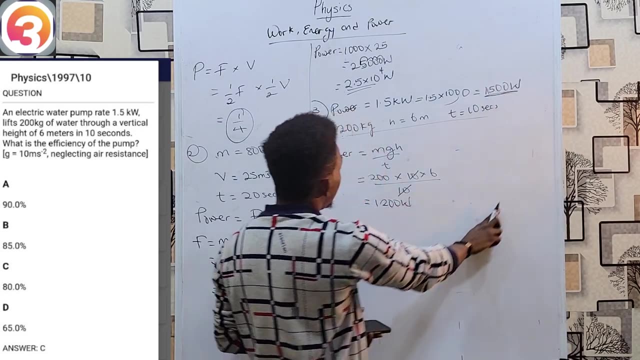 g, as usual, is 10, h is 6, over time 10, 10 cancels 10, and 206 is 1200 watts. that means, despite the fact that this pump is rated 1500 watts, instead we're expressing the power of 1200 watts. so how much. 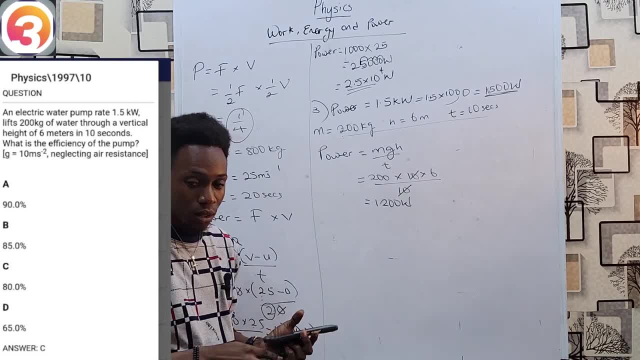 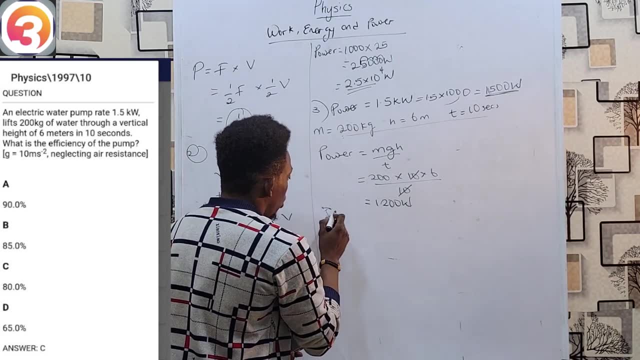 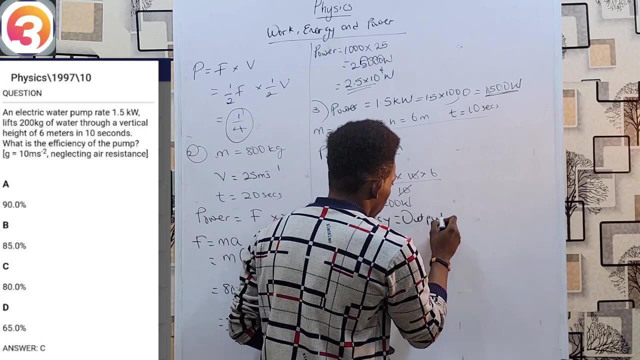 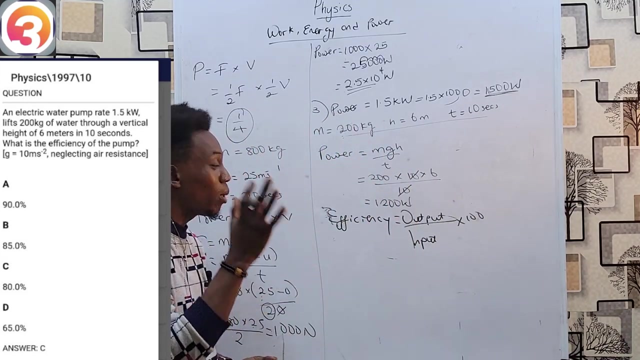 power, might we say, is getting wasted. to answer that question, all we simply have to look at this. now we know efficiency, or calculating weights. efficiency is always the output over the imputes times 100. that's the general form of efficiency, no matter the system. so the output is 1200. 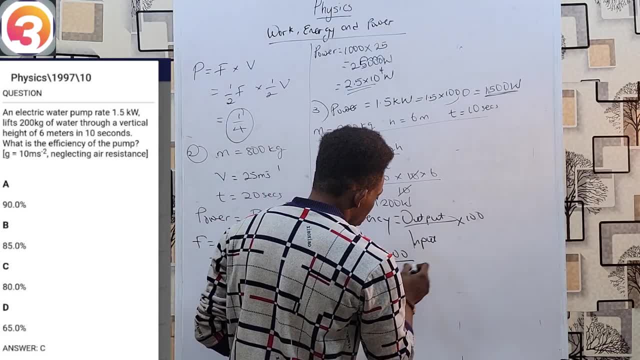 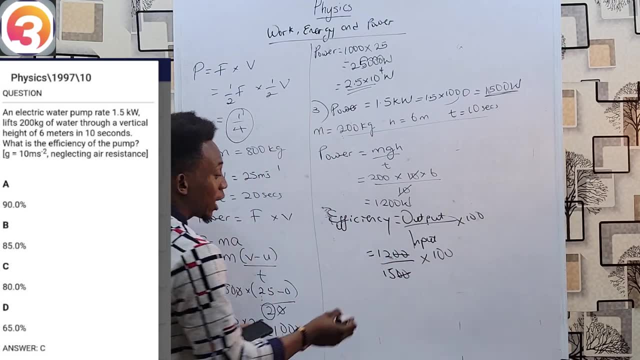 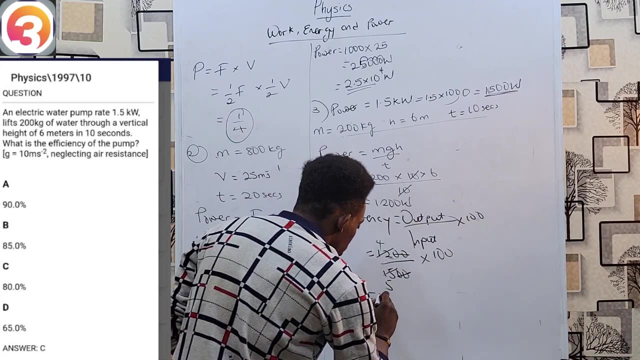 but the input rate in the actual rating is 1500 times 100. so zeros cancel zeros um. if you like, you could also say: 3 into 12 is 4, 3 into 15 is 5.. so you'll be having 4 times 100 400 over 5. 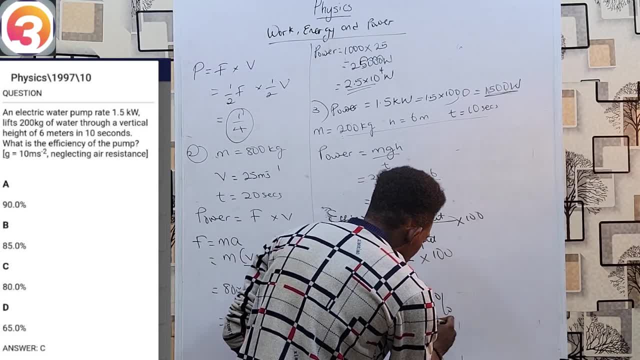 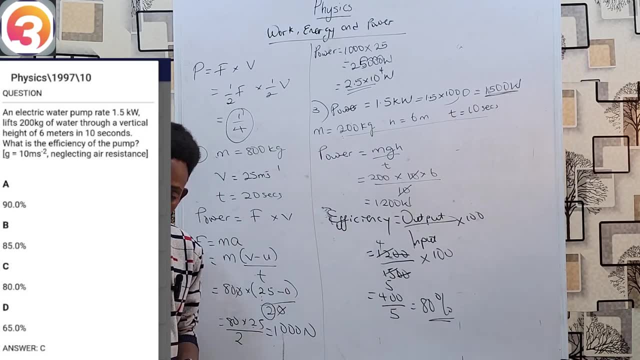 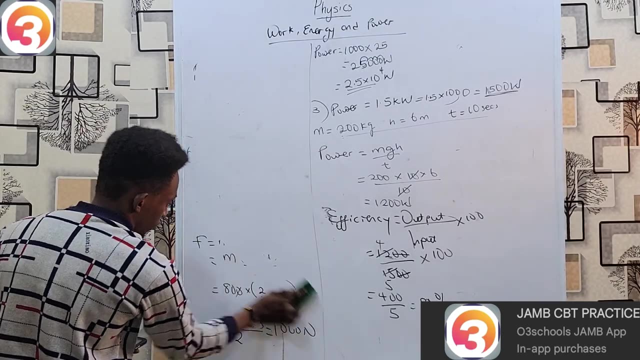 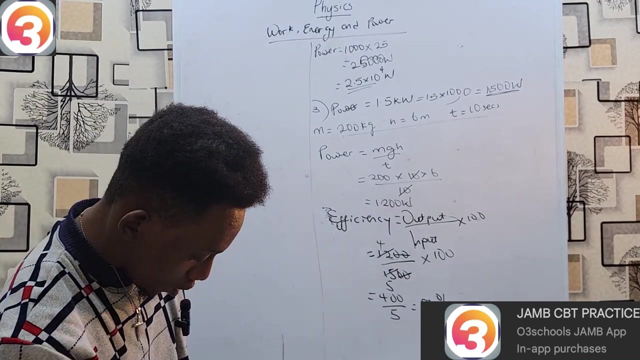 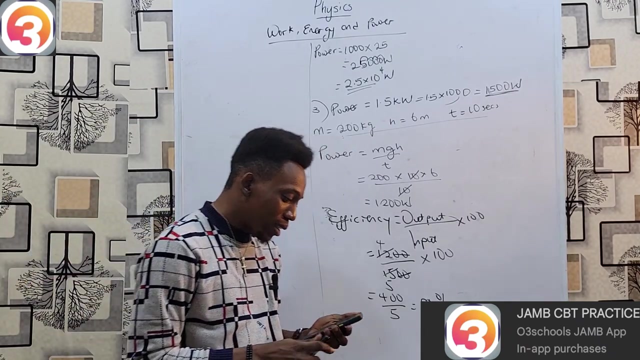 we divide this, you get 80 percent, which is our option c. okay, let's proceed even further and take a couple more examples. okay, um. now for this one we're looking at um question goes. this is, by the way, this is from 1998, question number nine, and it's 98, question number nine. 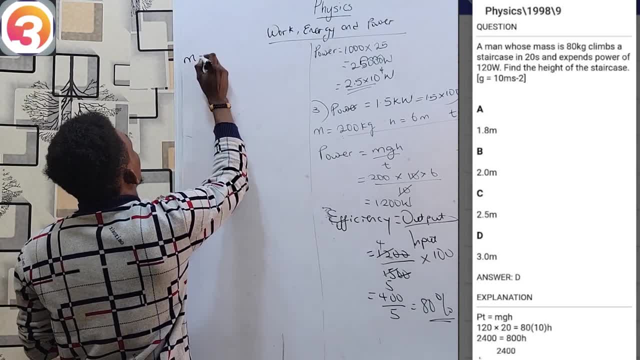 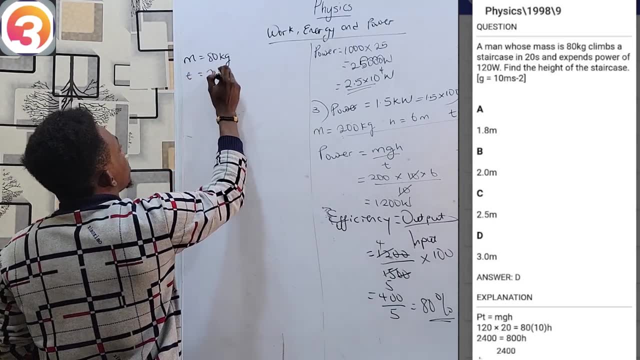 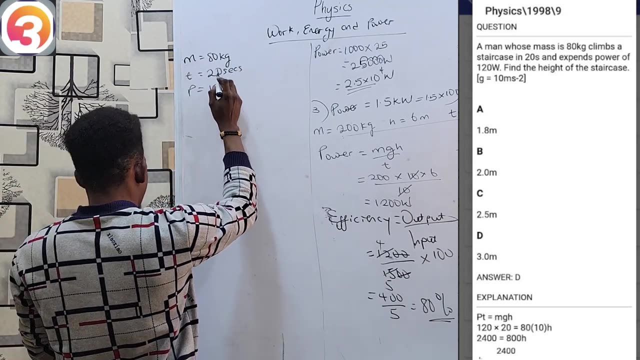 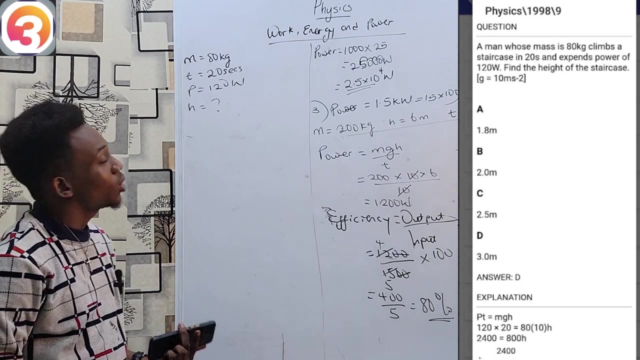 a man whose mass is 80 kg. the man whose mass is 80 kilograms clamps a staircase in 20 seconds. he claims of the staircase in 20 seconds and expense power of 120 watts. we have to find the height of the staircase. it's a kg climbing 20 seconds, 120 watts and the height? quite simple, as you know, based on what i 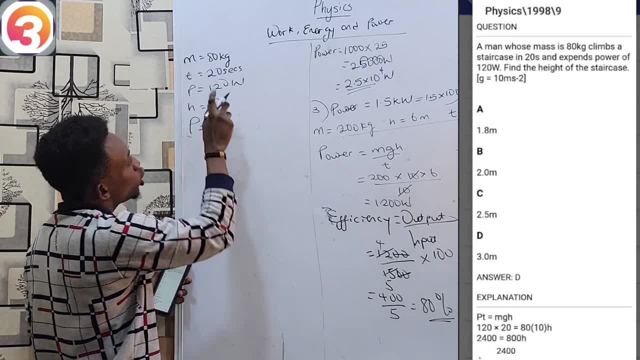 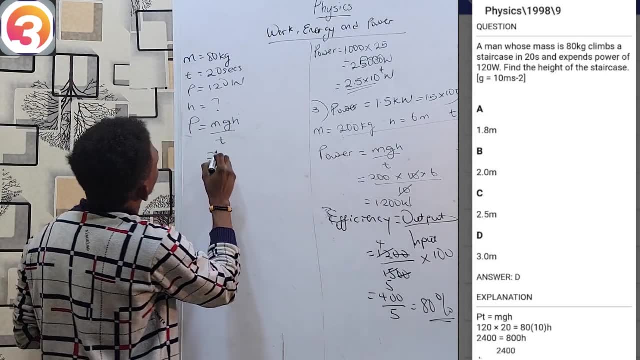 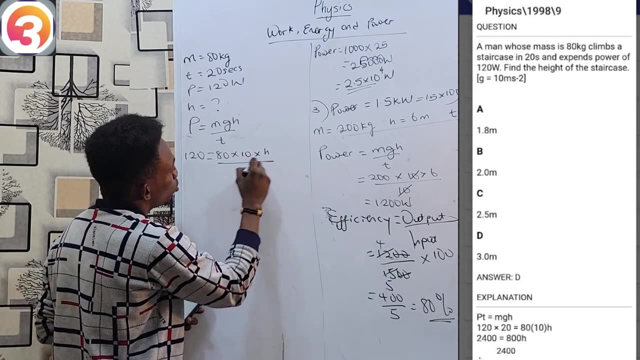 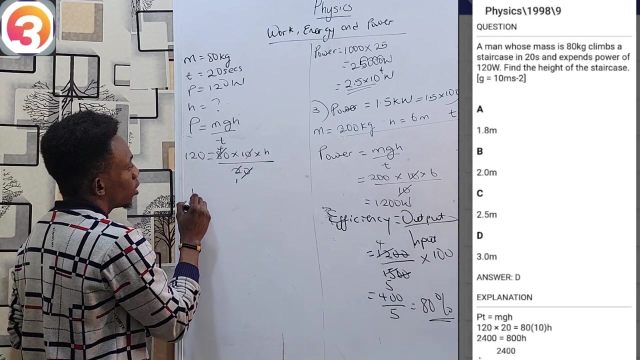 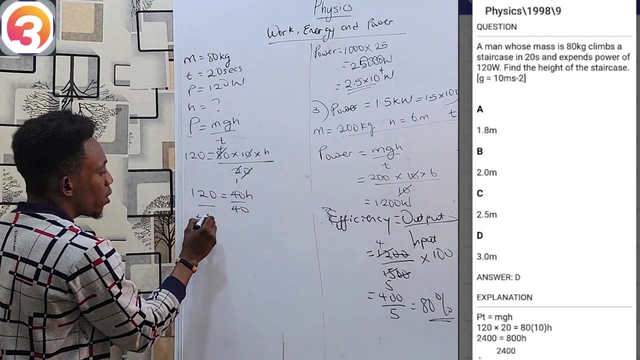 have, i know that my power must be energy if i'm climbing professional energy mgh about time to 80. 120 equals 80. g is 10 times h, if you do not know, over 20.. let zero, cancel zero. year one to year four. so 120 equals to 40, h over 40 over 40. so h equals to 120 by 40, which is: 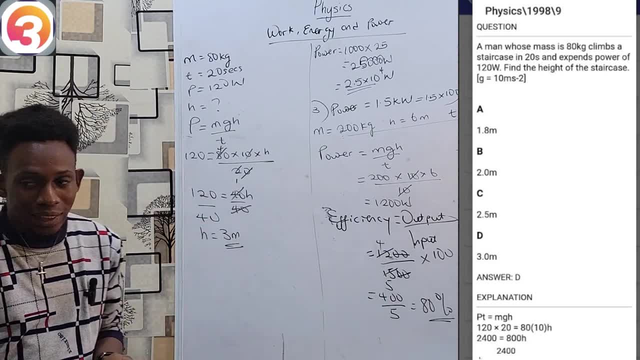 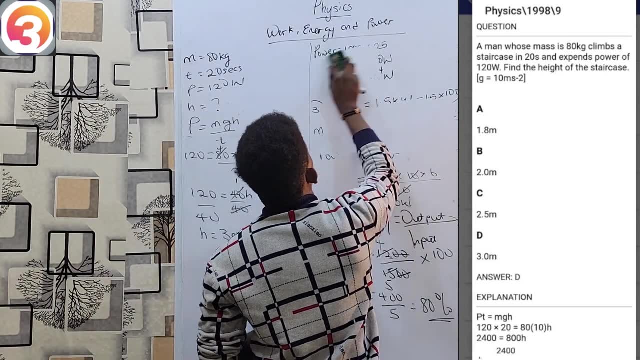 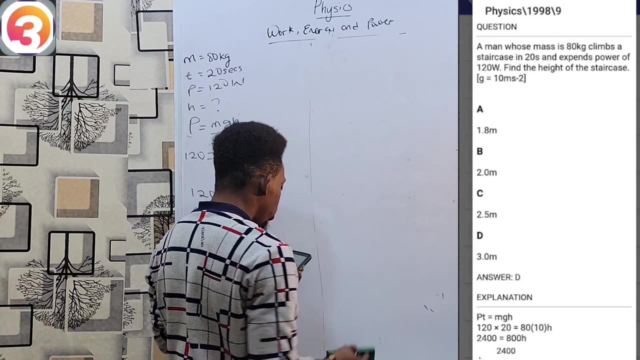 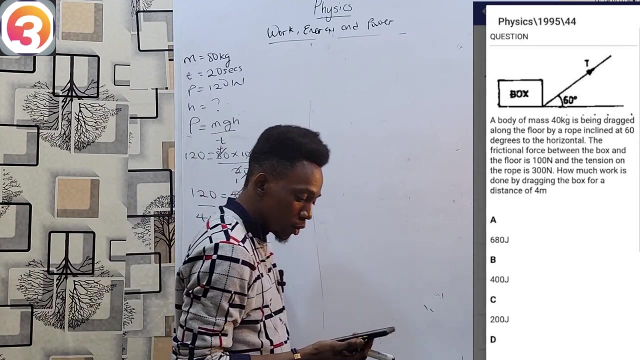 three meters, our option d. so you see, just keep your steps in mind and slowly, carefully, solve your questions. okay, the next question which i'll try our hands on comes from 1995, question 44. as again you can see in your app, this one states: by body of mass, 40 kgs being dragged along the road. 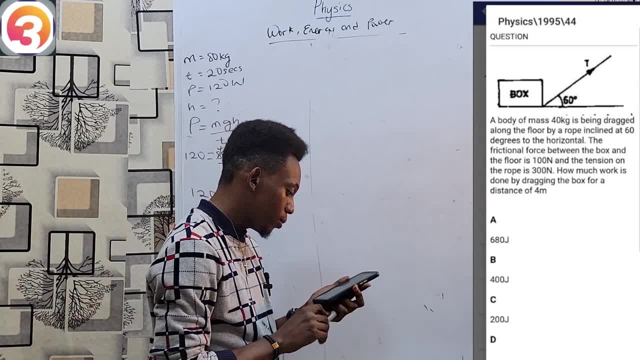 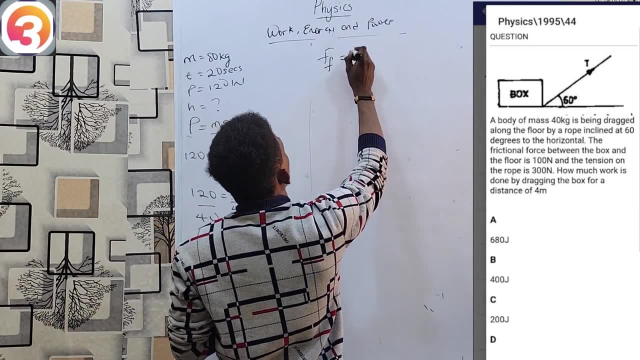 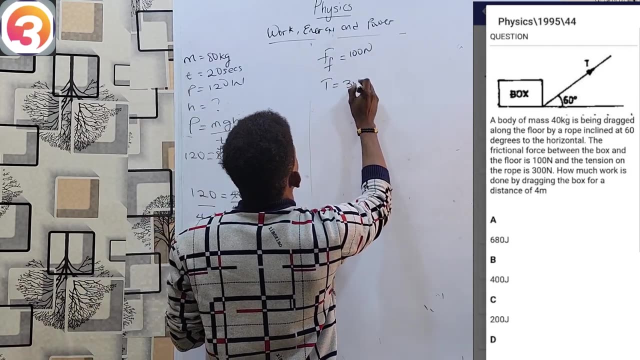 by rope inclined at 60 degrees to the horizontal. if the fictional force between the box and the floor is 100 newton, now fictional pulse of 100 newton and the tension in the rope is 30 degrees is 300 newton. we have to find out how much work is done by dragging the box. 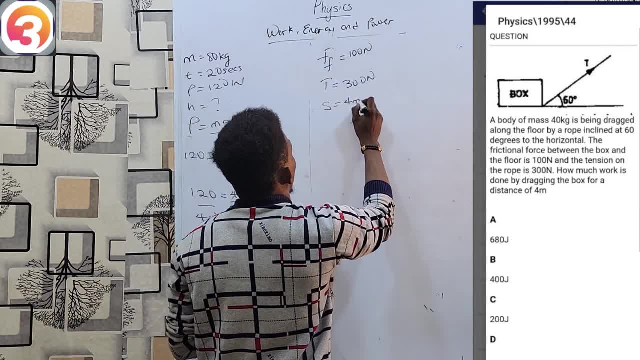 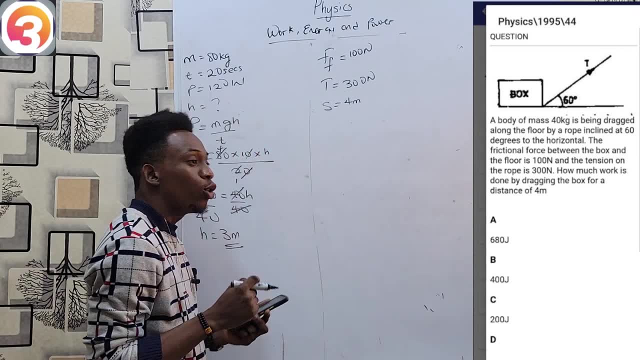 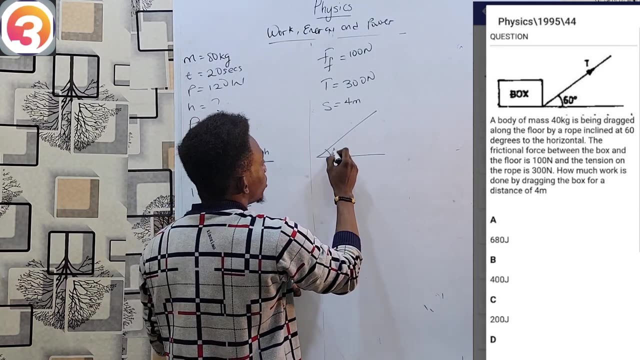 a distance of four meters. now the first thing we realize is that, from the diagram we can see in our app, this tension in the rope is not horizontal, it's at an angle, which means we have to resolve it and find the horizontal components. here is the degrees and here is the 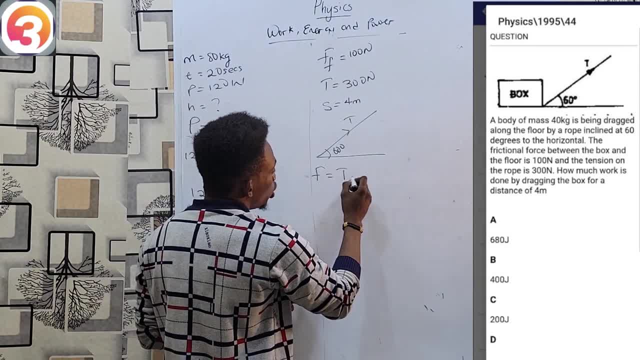 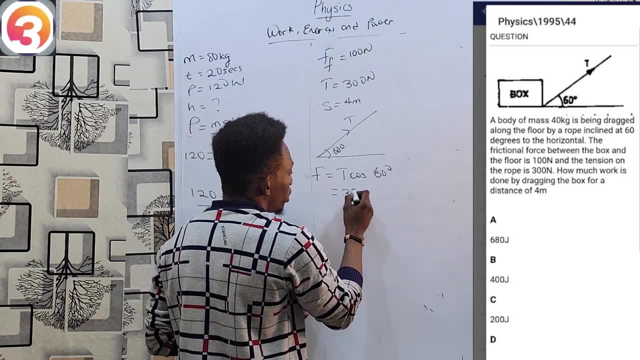 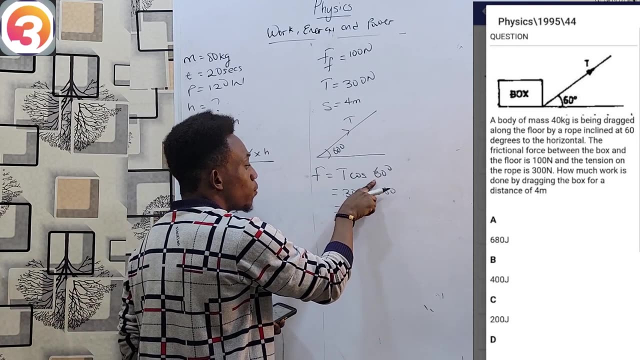 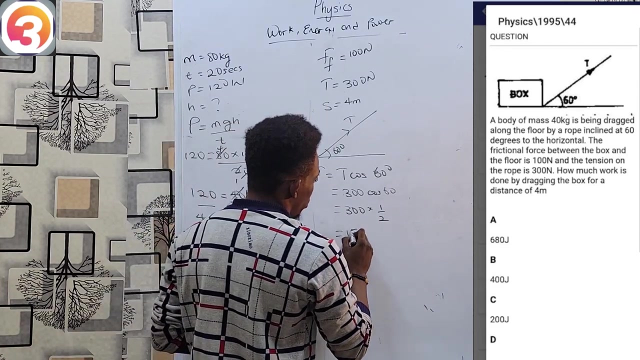 tension. therefore, the real force must be the tension, cos 60, and the tension is 300 cos 60.. and one more time why trigonometry is important. you have to know the value of cos 60, because cos 60 is simply 1 over 2, which means our force is 150. 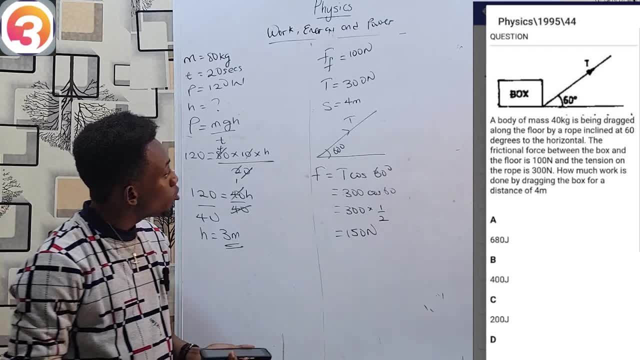 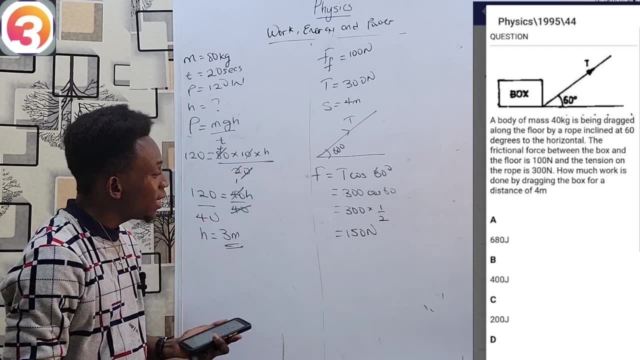 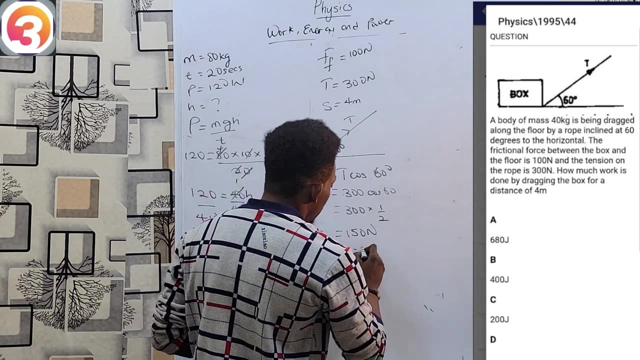 newtons. now, once we know this, we must then remember, based on the way i'm applying my force, my force is being opposed by friction, which implies that the true force dragging this will not be 150.. the true force, the net force, will be this force minus the frictional force. 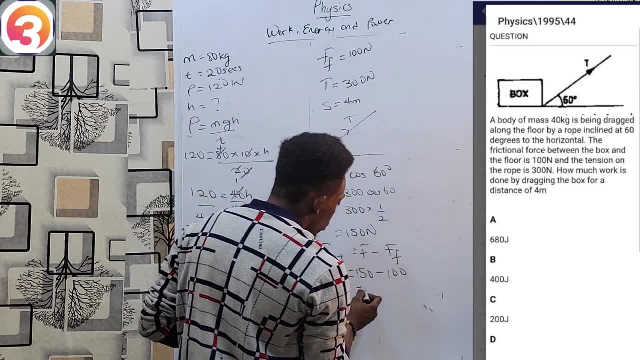 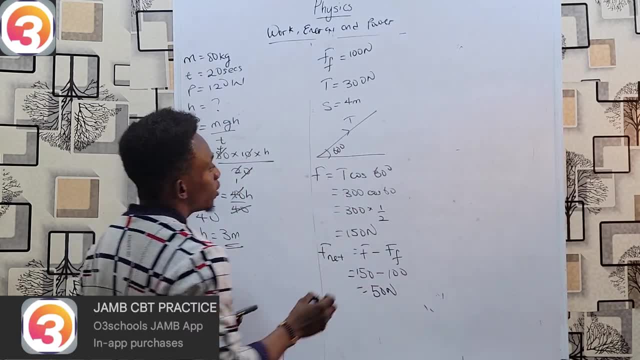 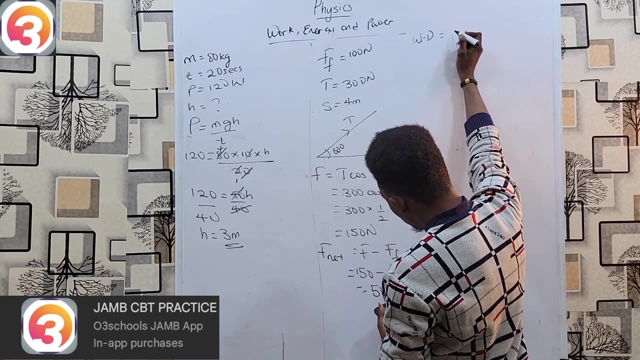 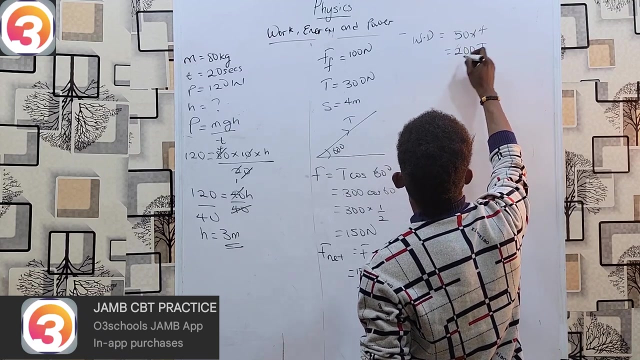 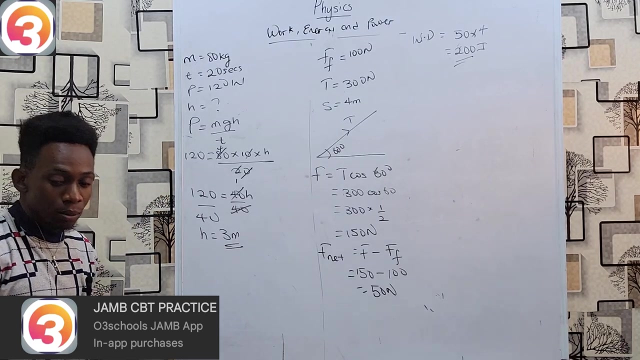 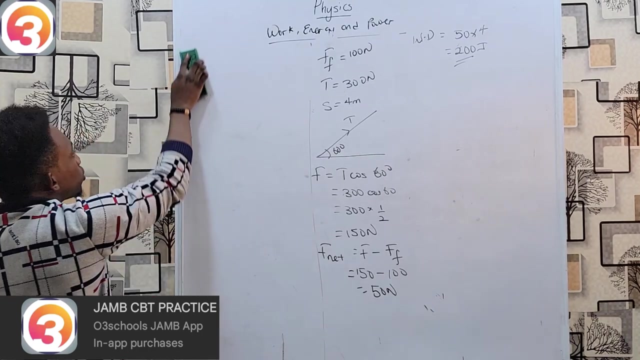 150 minus 100, you always have to overcome friction before you can move, so the force that will actually appear is 50 newton. therefore, if i'm going to move, ят need to know about the topic, that is, work, energy and power. now for this question. we have been told: 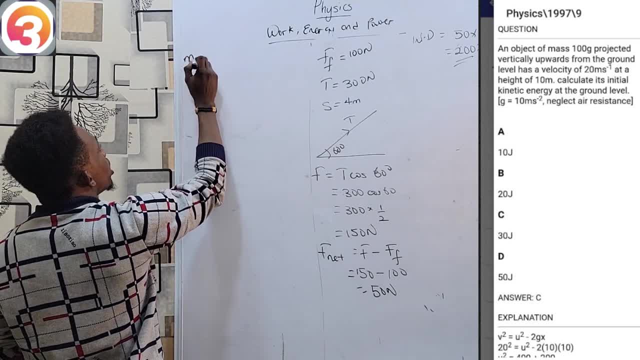 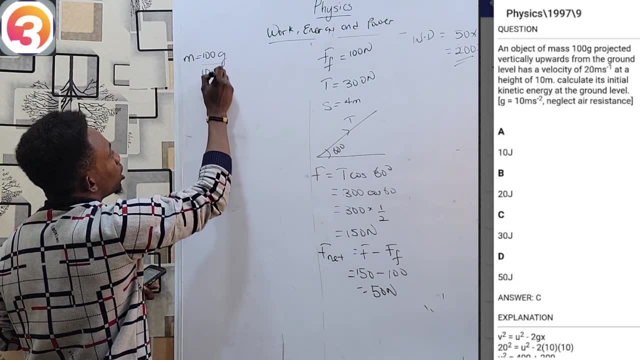 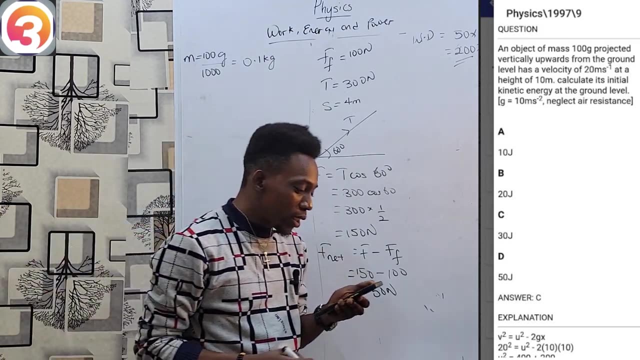 an object of mass, 100 grams. and here is one of the places where we need to remember conversion. 100 grams we do not solve in grams. solving kilograms to divide by 1000, 2.1 kg, okay. it is projected vertically upwards from the ground and it has a velocity of 20 meters per 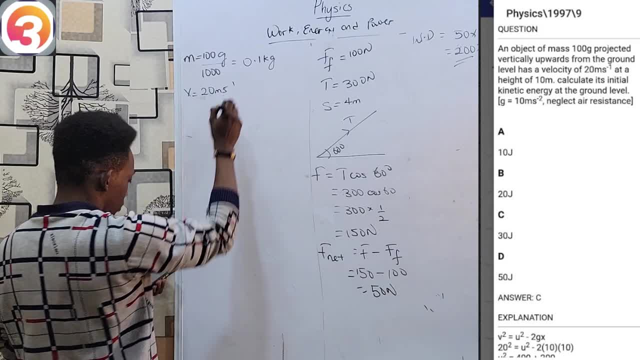 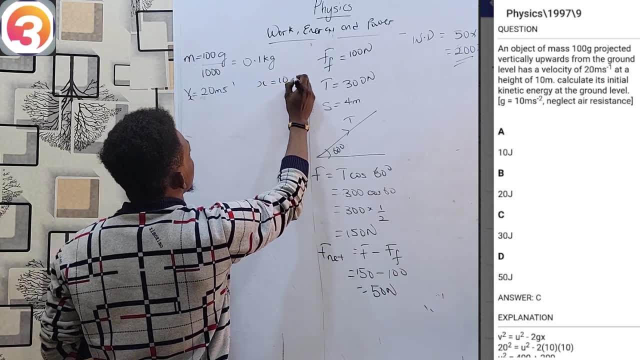 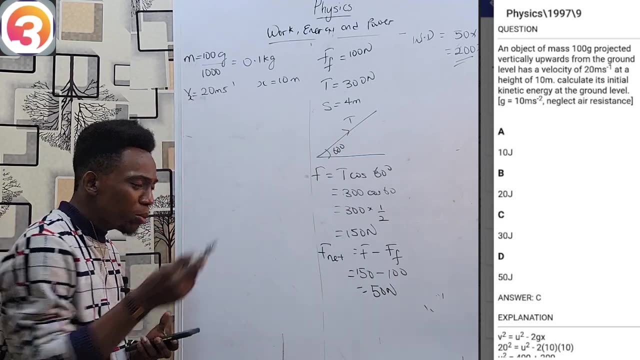 seconds plus equals to 20 meters per seconds at a height of 10 meters, at the height of 10 meters, but calculate its initial kinetic energy at ground level. now, if you remember the diagram we drew, we said: at ground level it has a velocity of 20 meters per second. and it has a velocity of 20 meters per second. 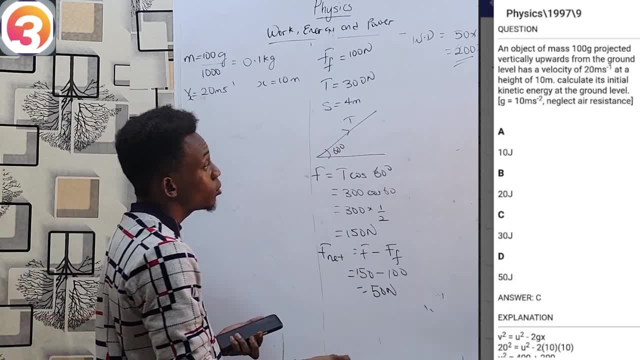 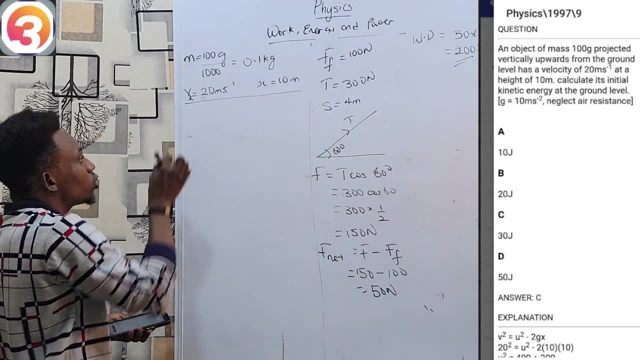 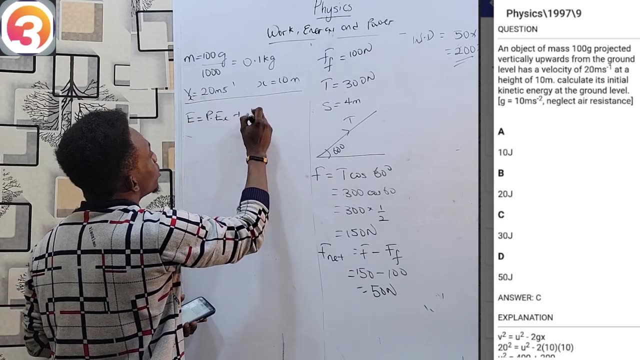 remember that static energy is maximum, while the potential energy is zero. what that must mean is that at this point x, where the height is now 10, and this is the velocity, if I also find the potential energy at this point plus this kinetic energy at this point, 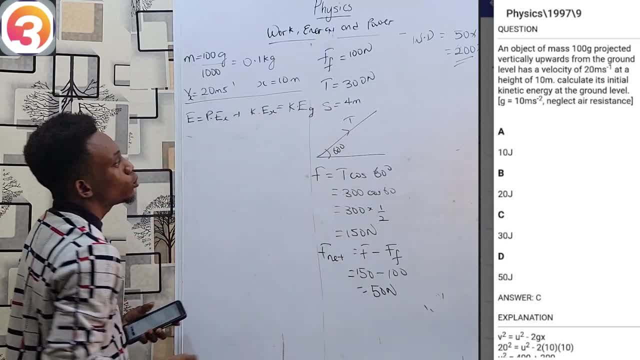 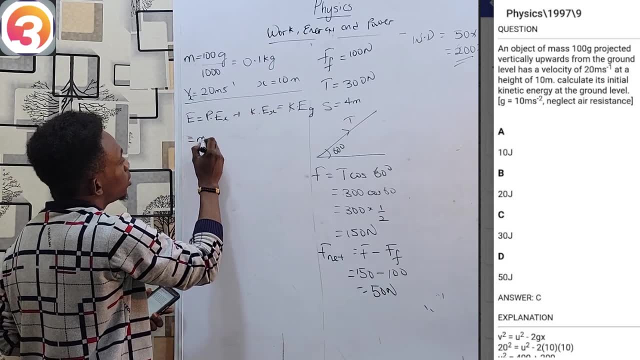 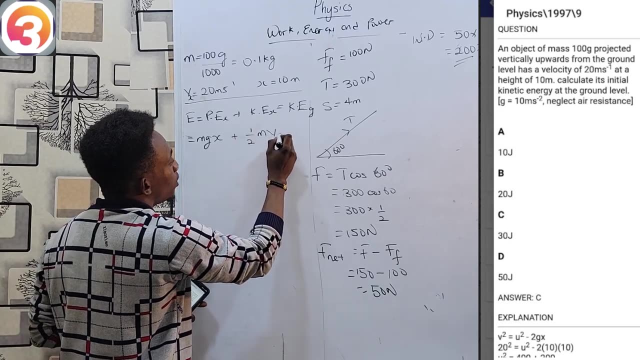 it will give me the kinetic energy at ground level. don't have to do much solving. all i así have to do is that Potential energy at set point must be mgx and kinetic energy at set point will be 1 over 2 mvx squared. 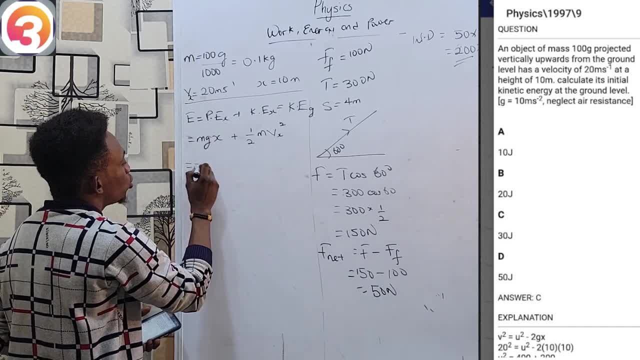 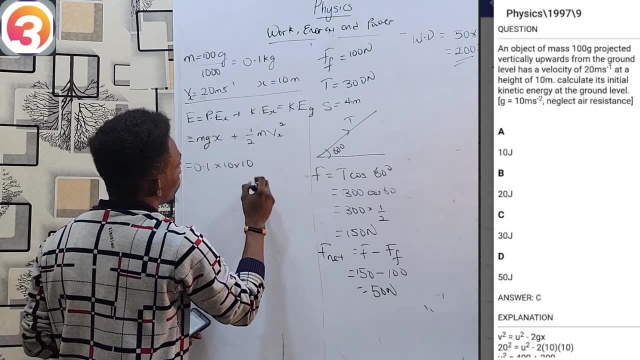 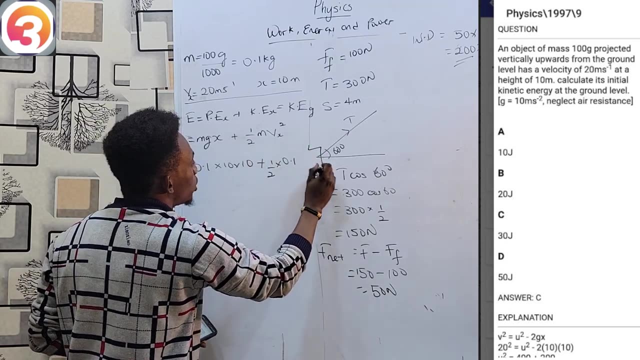 So, going through it, m is 0.1, as we have up here, g is 10, as usual, and x is 10 plus 1 over 2 times m remains 0.1, while my velocity becomes 20, so 20 squared. 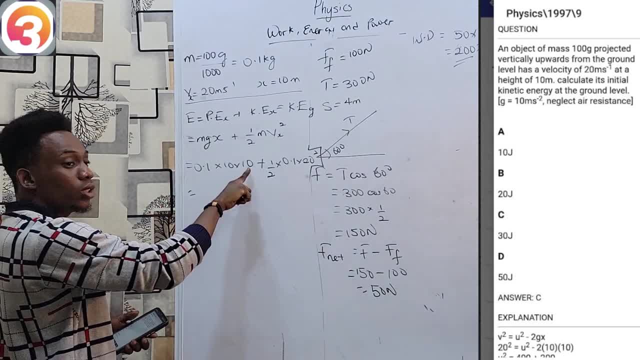 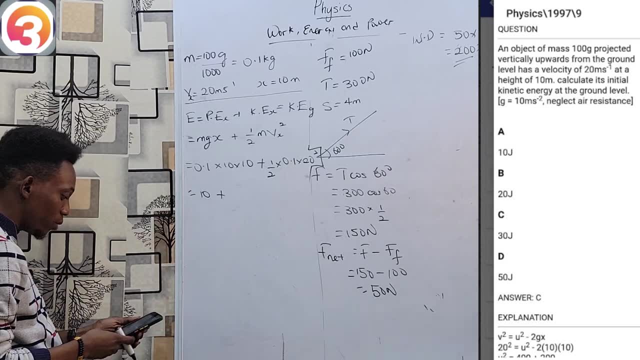 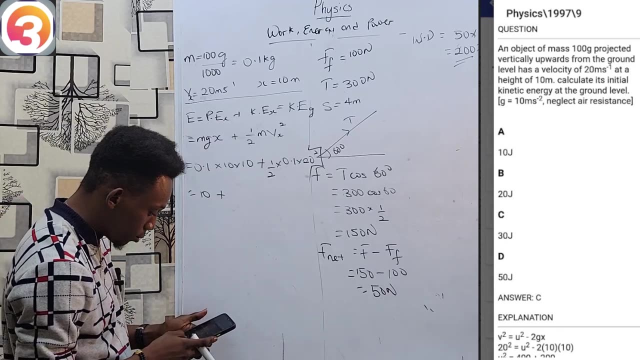 So calculator 10 times 10 is 100, 100 times 0.1 is 10.. While over here personal calculator there, if you can't solve that with your head to avoid mistakes, we know that that will be 0.5 times 0.1 times 20 squared, which is 20 times 20.. 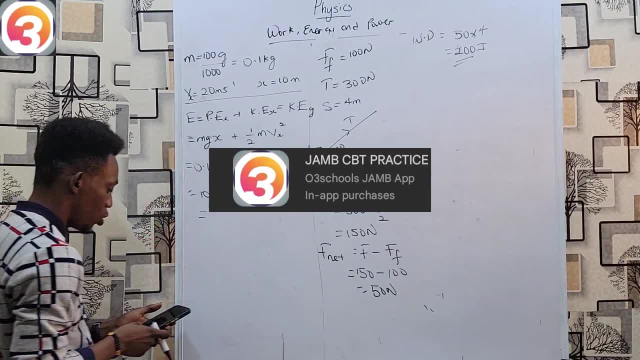 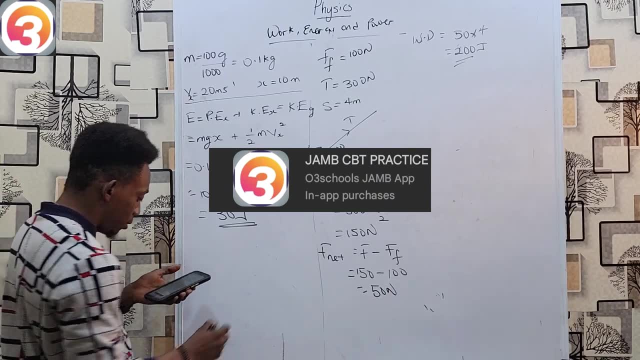 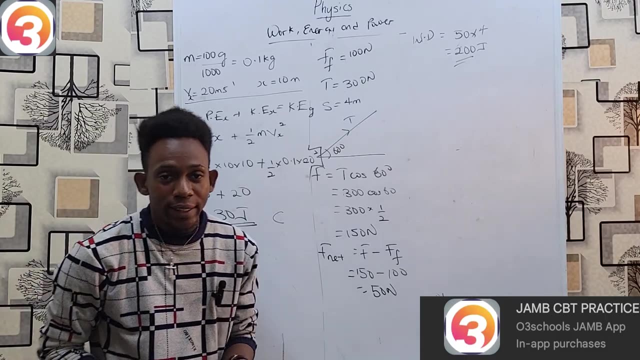 And that gives 20 joules. So quite simply, 10 plus 20 equals 30 joules. Option C: the kinetic energy at that point is 30 joules And at this point I'd like to say thank you for attending this class and listening to us. 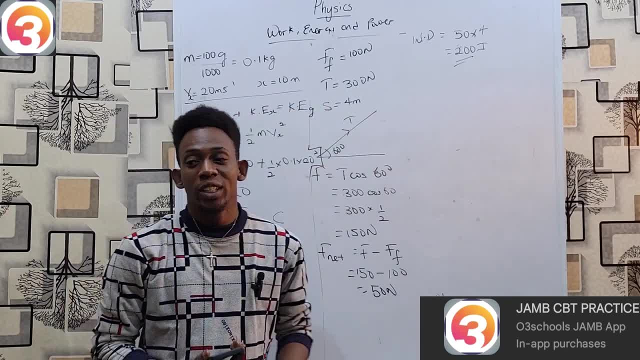 Please remember both ways. close, jab up. My name is Kaderu Ikane and thank you for listening. 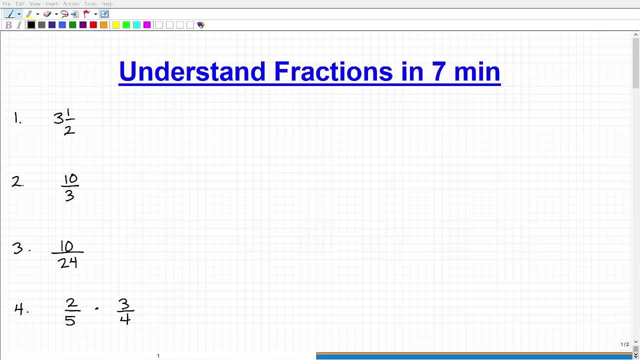 Okay, so the goal of this video is to get you to understand fractions in about seven minutes, so let's see if we can do it. really Obviously, am I going to get you to completely master fractions in seven minutes? No, I'm expecting that you've studied fractions before. 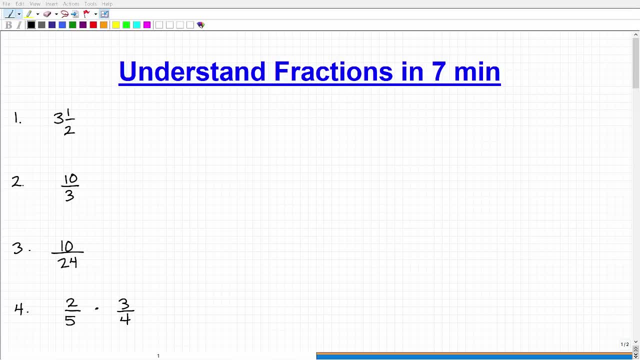 So this is going to be like just a quick review of the basic functions with dealing with fractions, but we are going to cover pretty much the Whole scope of most common problems that you have when you're working with fractions. okay, So I've got seven problems. Let's start with the first one. all right, so three and one half. This is called a mixed 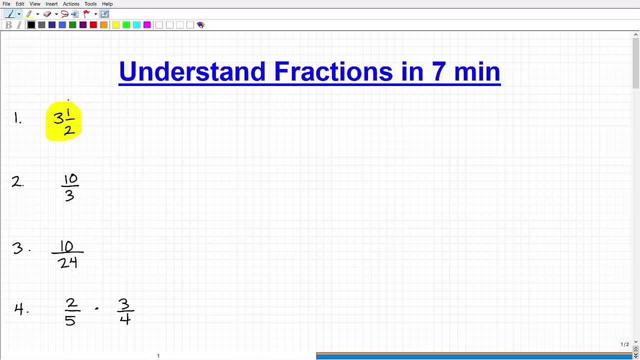 Fraction: okay. so if you have a number and a little fraction next to it, That's called a mixed fraction. so we need to be able to write a mixed fraction as an improper fraction. That's a fraction like down here, like 10 over 3. 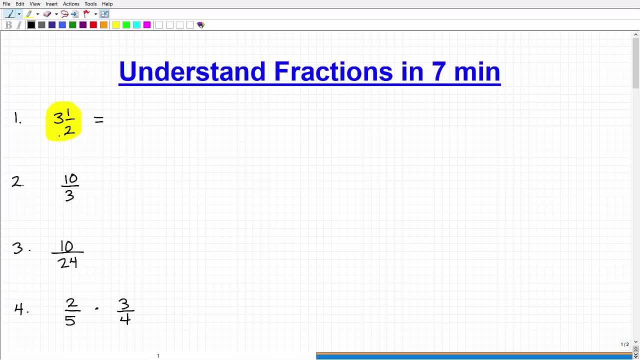 So the way you do that is just you take this bottom number 2, You multiply it by 3 and then we're going to add the 1, so you probably remember how to do that. so that's gonna be 2 times 3, That's 6 plus 1. is going to be 6 plus 1 at 7 over 2. okay. 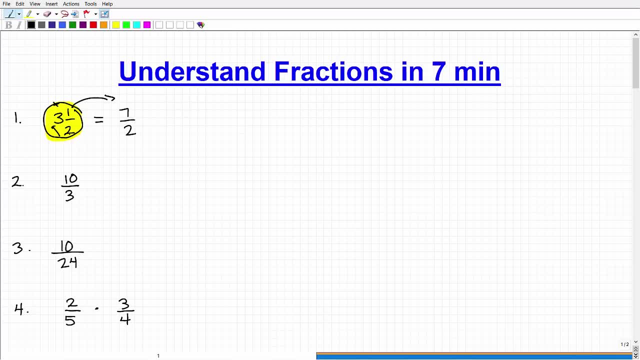 So we need to be able to take mixed number fractions and turn them into improper fractions. now We also need to- let's move on our second problem- take Improper fractions and write them as a mixed number, so that what we do there is: we simply go ahead and just divide.